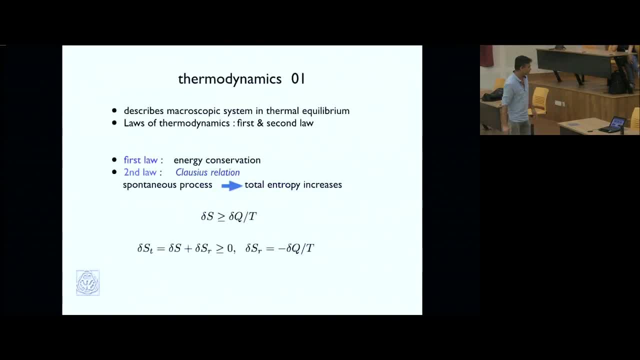 systems I have in mind. But before that, a little bit of recap of thermodynamics, whatever I'm going through. So first, things are okay. so we know the first law, second law of thermodynamics, So energy conservation, And then in macroscopic second law, we know that entropy, production of 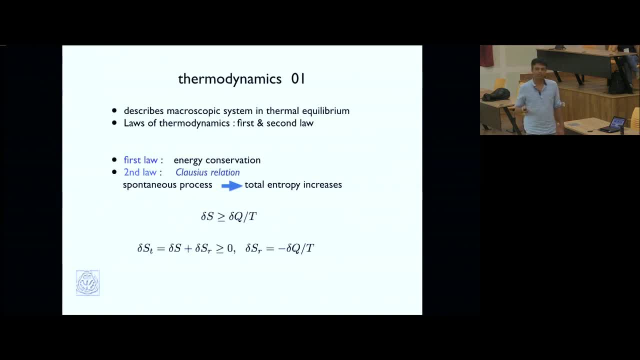 the system plus reservoir, And if we write it down in that fashion, so the reservoir entropy production is supposed to be the heat. So in my notation it's the system, whatever it is, absorbs the heat, increases its energy. So heat released by the reservoir to the system, or so. 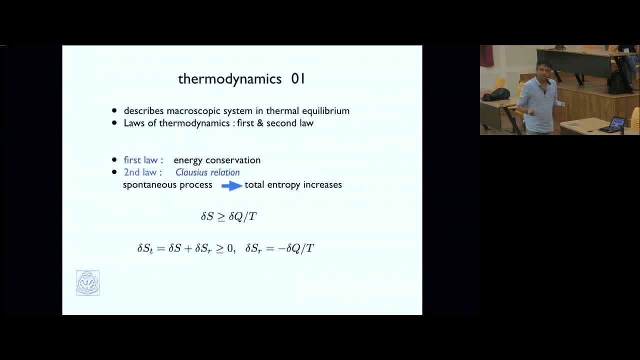 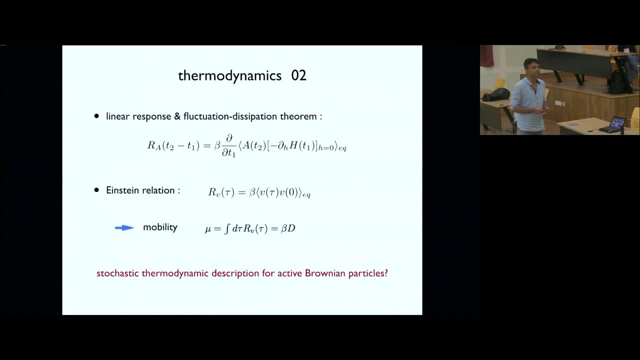 that's the entropy production in the reservoir. So that's what. and the second part is we normally look at linear response to look at and look at the relation between the linear response and the fluctuations in the system. that's in equilibrium. But now I'd ask this question that can I develop a stochastic thermodynamic description? 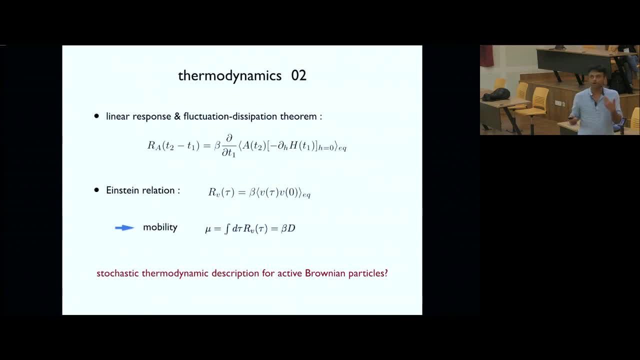 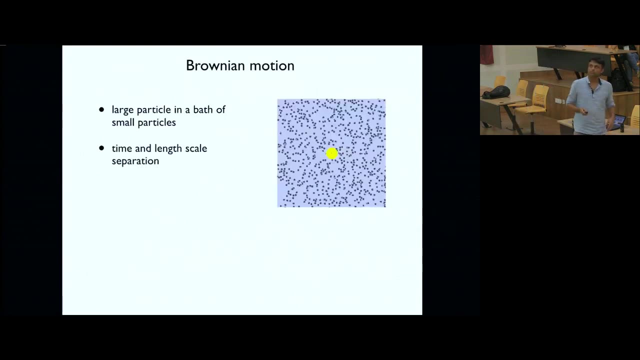 Of course we can, For active Brownian particles. so taking the stochastic regimes of thermodynamic quantities and also looking at response function. Okay, so, before I get into my system, so to set up the language, so we'll be looking at Brownian. 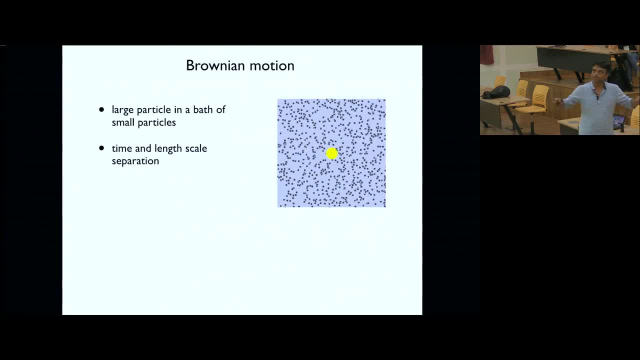 motion. So Brownian motion means that I have larger particles sitting in a bath of smaller particles And then there is a length and time scale separation between the large particle motion and the small particles, And so then, if you look at this, the larger particle will undergo random motion. so 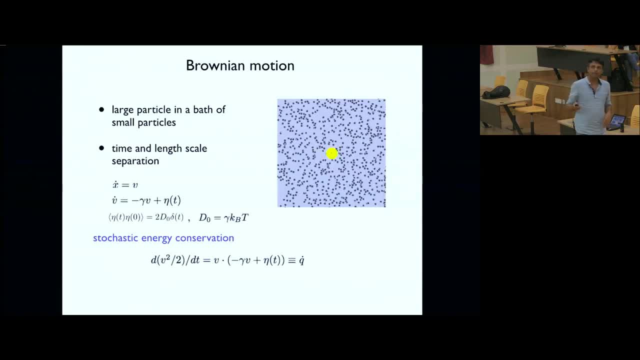 movement in this bath And then one can write down the equations in terms of the position and the velocity, where this part is the energy, this part is the forces coming from the heat bath. So this is the dissipative part and that's the fluctuation, and I obey the fluctuation. 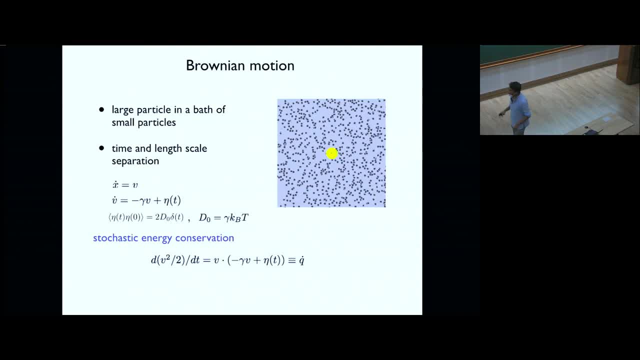 dissipation relation. So if I switch off all my activities, my system should go back to my equilibrium system. So and then, starting from this equation, one can just multiply with the velocity, write down an equation for energy conservation, So it just has kinetic energy. 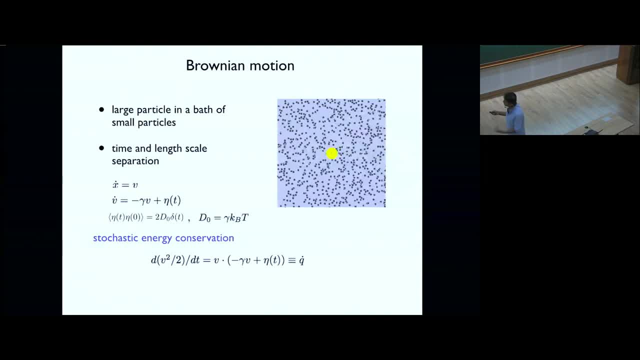 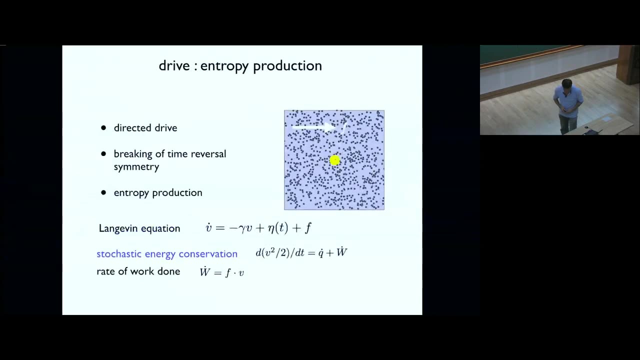 which will be now given by the heat absorbed by the system. by the system means the single bead floating in the heat bath. Okay, So, yeah. So the simplest way We can drive the system out of equilibrium is to put some external force on the system. 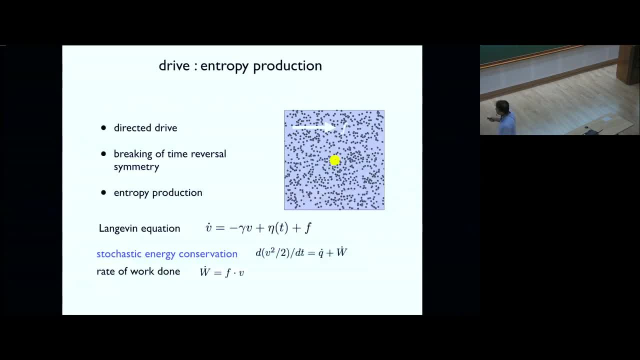 So then one will give a directed force and write down the line given equation in presence of this directed force and that changes the stochastic energetics to energy conservation will be now given by the total heat absorbed by the system and work done on the system. 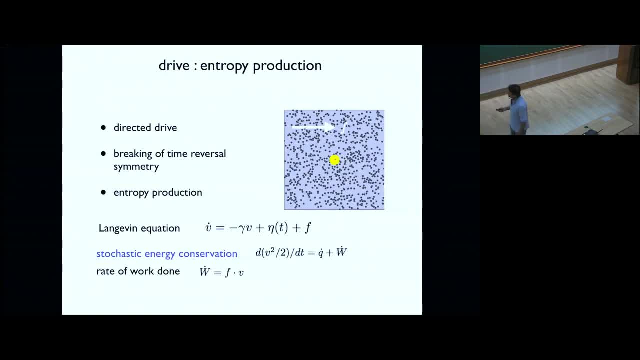 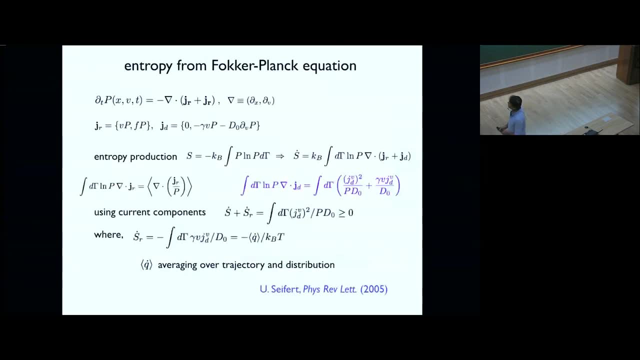 So that's the rate of work done. So I'm just using standard, well-established notions, and much of these notions are established by Udo, and so he has several review articles. I particularly like this one-page argument in that. So there are two ways. 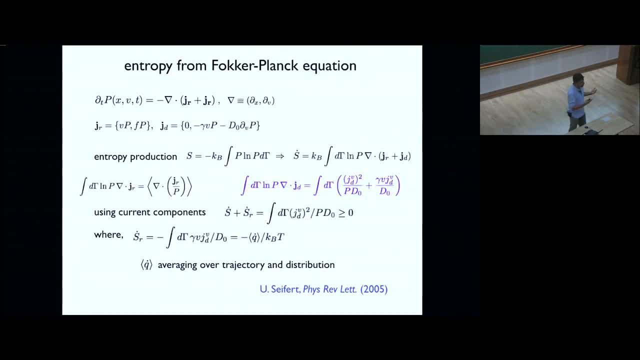 One can now if I go out of the energy conservation picture and then look at the entropy production. So if I drag the system out of equilibrium, if the time reversal symmetry is broken, the system should be producing entropy, and then we can calculate entropy either from first writing down an equation. 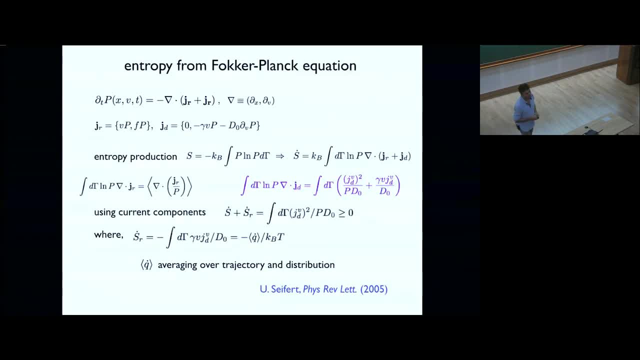 for the probability distribution, a Fokker-Planck equation, or you can also look at the probability of forward and reverse trajectories and then taking a ratio of these trajectories and defining entropy from there. So I'll just give you a brief outline of this description before I get into my system. 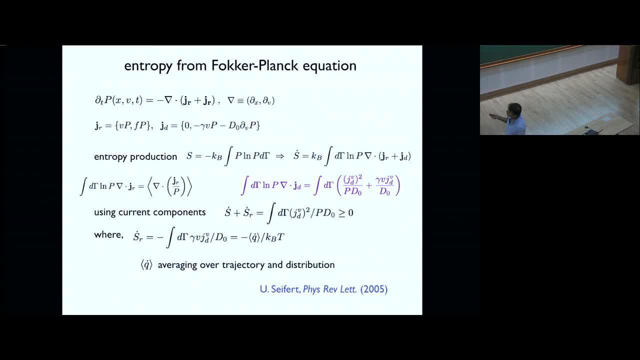 So we write down the Fokker-Planck equation. I am writing it down in dividing the total current into reversible. So should be dissipative JD reversible and dissipative part of the current. And then this divergence, this gradient operator stands for the positional and velocity differentials. 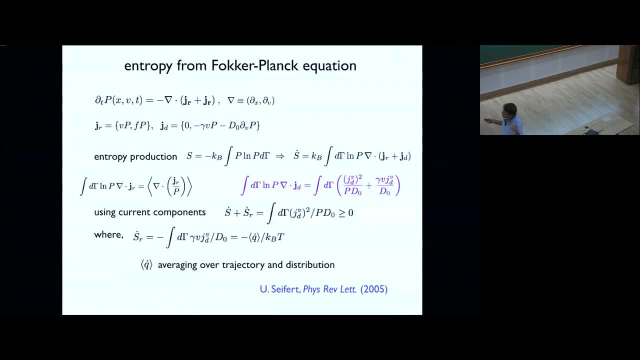 And the reversible current part is given by: first is the velocity of the particle, Second is this external force which we assume that Under time reversal this doesn't change its sign- and the dissipative part of the current. So for positional side it has nothing but the velocity component. it has two parts. 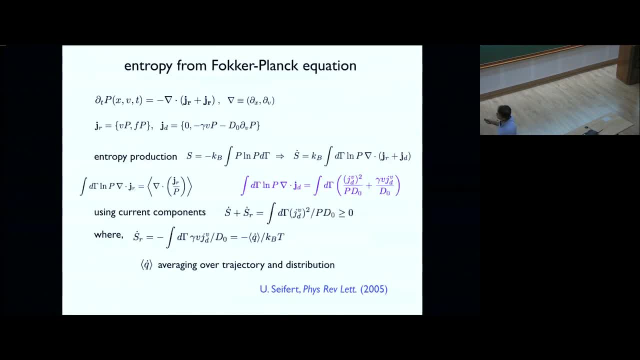 One is coming from the dissipation gamma and then the other part is from the stochastic forces And then one can write down the total entropy in the system in terms of integration over DX and DV. So this is the space integral and write down a time derivative of this entropy production. 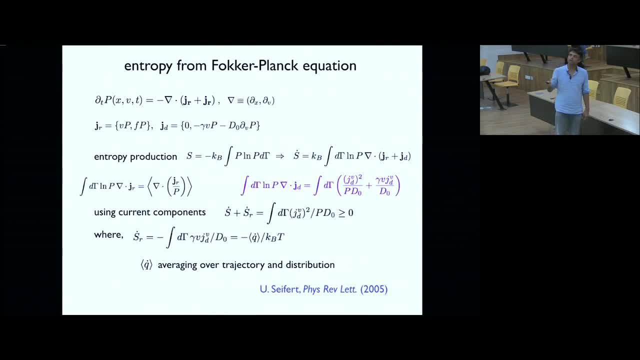 So entropy time derivative, which is the entropy production, then can write this down in terms of del, del T of P, plug in this relation a couple of steps of algebra. We can write it down as: So first is log P and divergence of these currents and then performing a couple of steps. 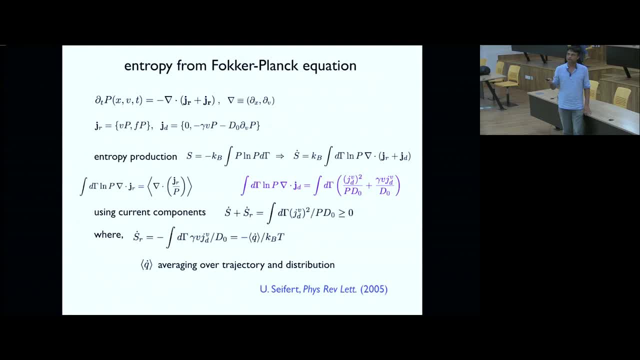 of algebra, You can separate it out. So one part is that log P- divergence of current. We can write it down. We can write that down as a divergence of reversible current divided by the probability and average over that. So it means that this is P D, gamma, integration of this. 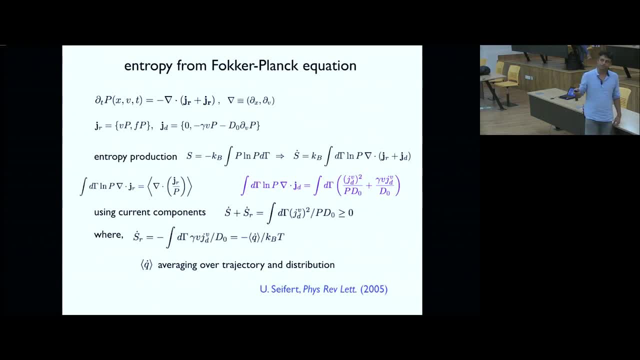 So this quantity, of course, within the system this goes to zero. Trivially, this goes to zero because this is a derivative with respect to X on V. So that will give me zero And this component itself is zero. So that's trivially zero here. 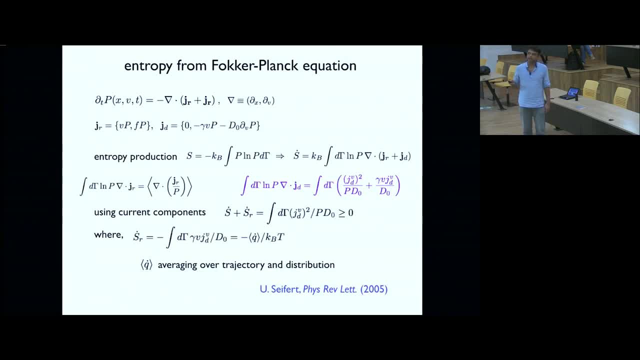 And the dissipative current. if I look at that part, one can write that down in terms of one part which is always positive Dissipative current. I'm looking at this. velocity component means this part minus gamma V P, minus D, zero del V P, that part here. 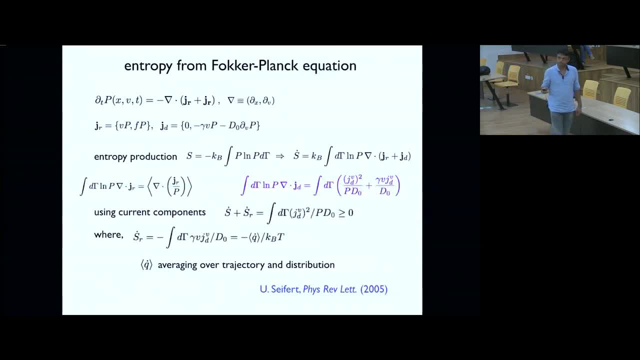 So that's always positive. And there is this extra bit, And if I take this extra bit to the left hand side in S? dot, plus this extra bit that the whole thing is greater than equal to zero, And this extra bit, we can then show that this extra bit is like a heat. 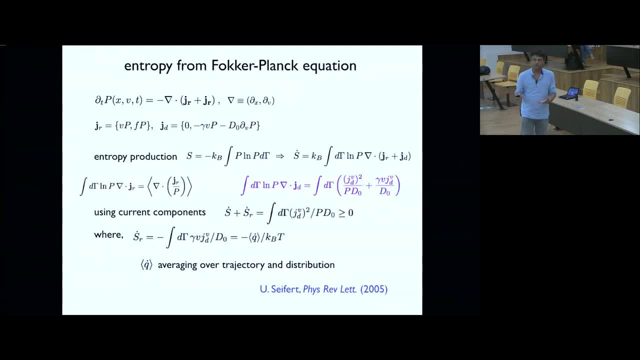 So like the entropy production in the reservoir. So that's Q dot by T. So I have this K B sitting here. So what we are getting is that this is a Q dot average average over trajectory and distribution, as nicely shown in this article. 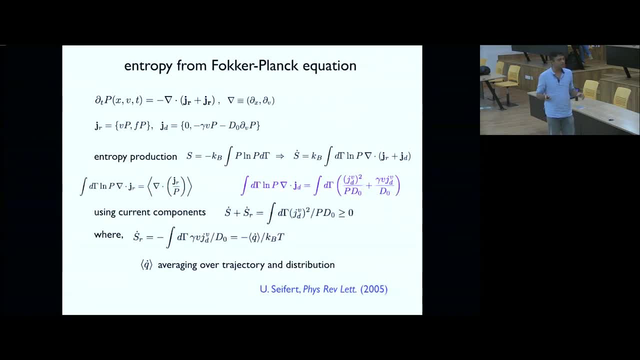 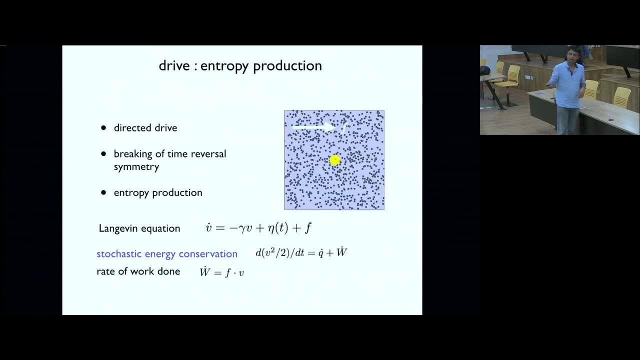 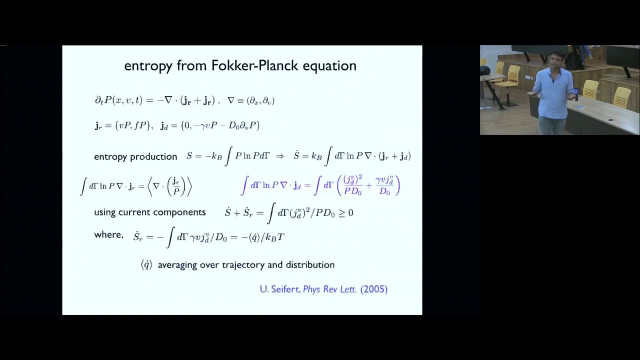 You can write this down: the reservoir heat production as an average over this Q dot, where the Q dot itself is the heat production as we have seen from this relation. So V times minus gamma, V plus eta, So that's the work done by the reservoir. 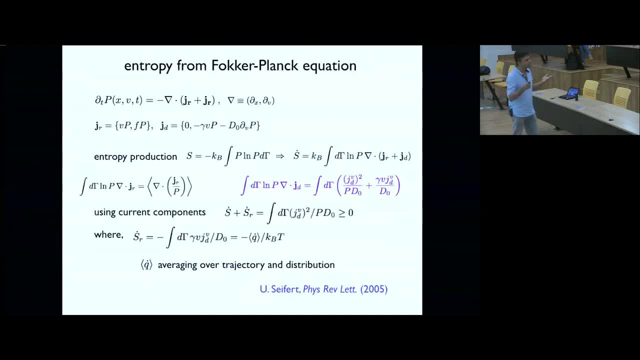 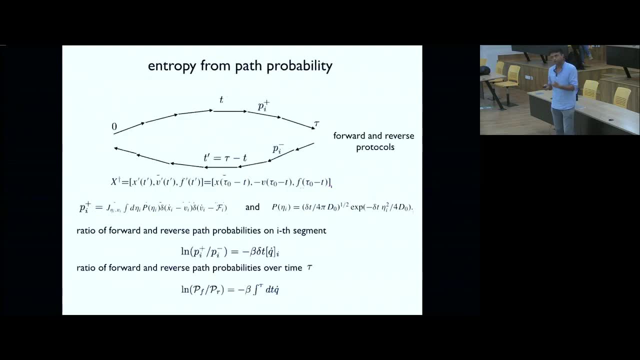 That's the heat production And that's in sync with the Clausius expression of the entropy production in the bath. So you can do that From the time forward and time reverse, path probabilities as well. So what we do is that I'll just describe this. give the outline. 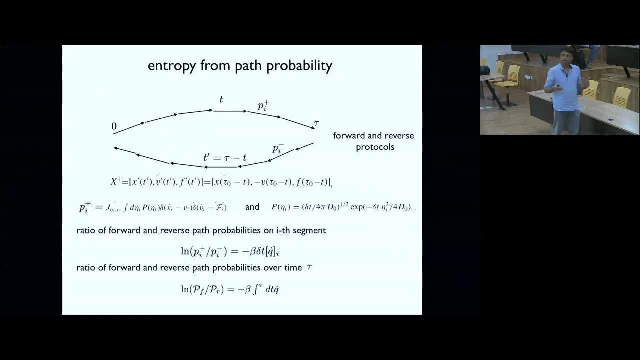 So if I take any trajectory, so under external drive, still the system is under external drive. I start with the probability distribution at time equal to zero and evolve the system up to time equal to tau And the system evolves and I can look at the path. probability distribution of the system. 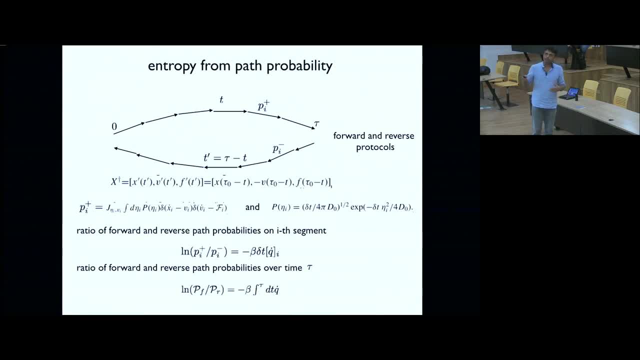 as it moves forward. So that thing for it. then the whole path. I can chop it up into small segments over some time. steps delta t, simplifying this whole path. integral, And let's say that on an is segment, this probability is Pi plus. 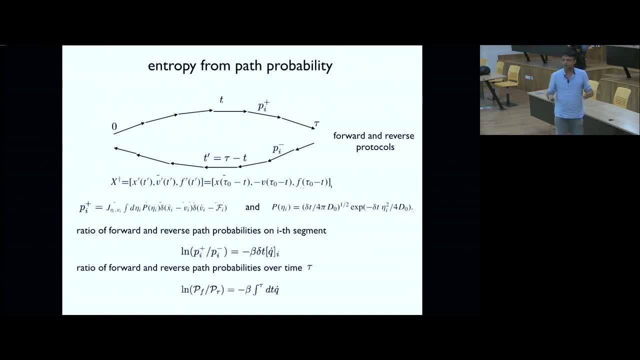 And then after this propagates in the after time, forward propagation. let's assume that the system goes to a final state and from the final state defined by this probability, final value of the force could be some f at tau. So what is the probability of system? 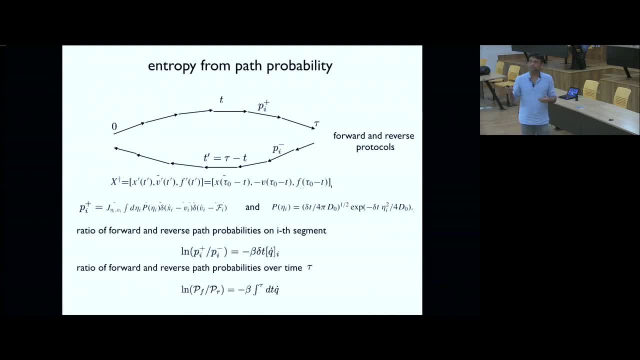 So I start from another configuration of the system which obeys this probability and then reverse it back. So this reverse trajectory, So reversal means that positions doesn't pick up sign. Velocity is odd function. picks up a sign. Force is an external quantity which doesn't pick up a sign. 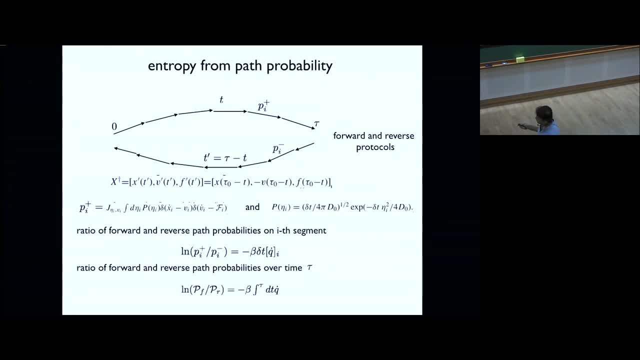 So you put this together, then you can write down the probability of this forward path, which will be apart from a Jacobian, which will be given by the probability of the reservoir noise, eta i, which we assume to be a Gaussian noise and which obeys then in presence of 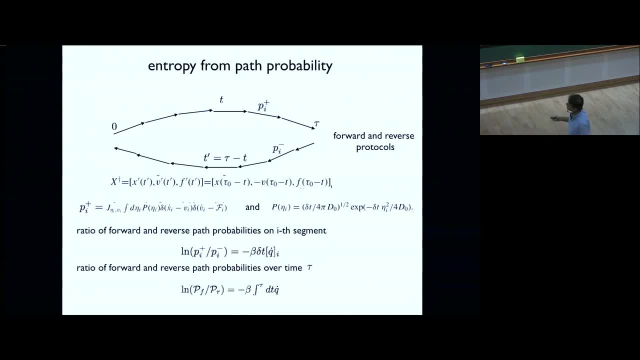 this constraint that they have to follow the equations of motion. So if one does this calculation and calculates the forward and reverse path, probabilities and ratio of that on this ith segment you can write it down as minus beta, which is one by kbt times delta t. 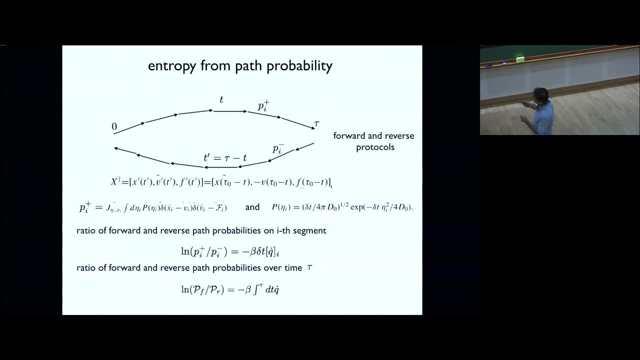 the time step over this segment and heat produced, heat absorbed from the reservoir q dot at that ith moment. Then for the whole trajectories, you can write it down as an integral. so multiplication of this whole thing. So that will be written down as an integral. 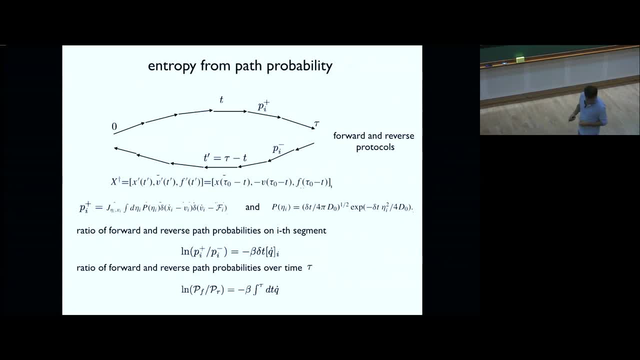 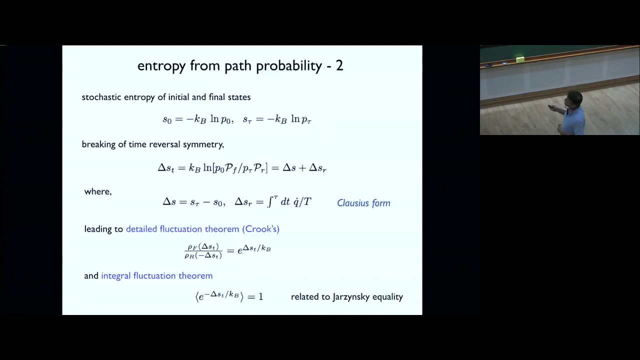 over the whole time: evolution, tau, dt times, q dot, where again the q dot is really the heat production, heat absorption, as we have seen from the first law. Then one has to also take into consideration the entropy in the initial state, entropy in the final state. 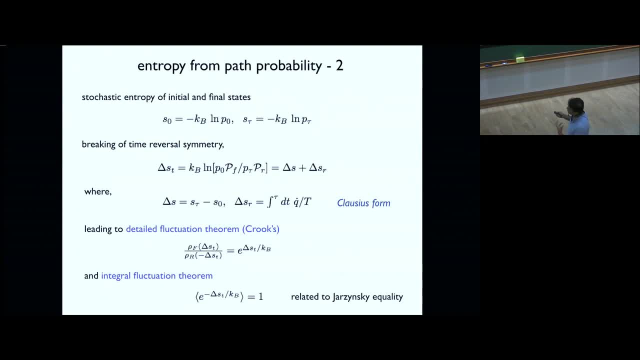 so the stochastic version of this entropy and then you club them together. the total entropy production will be given by the entropy change in the system, which is given by the difference s tau minus s zero and then the heat entered. production by the reservoir. 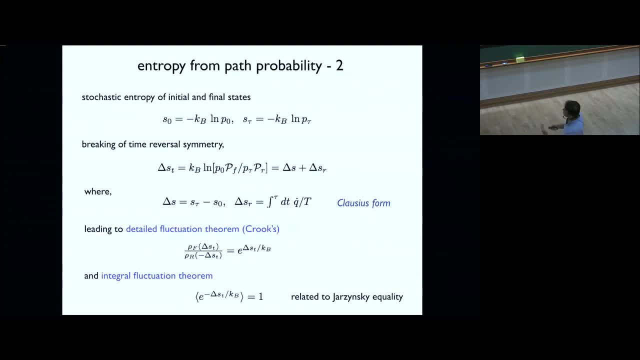 during this transition from the initial state to the final state, which is given by the total heat absorbed from the reservoir. So this should be a minus n minus q dot. So then one can show, using this relation, this forward probability and reverse probability ratio. 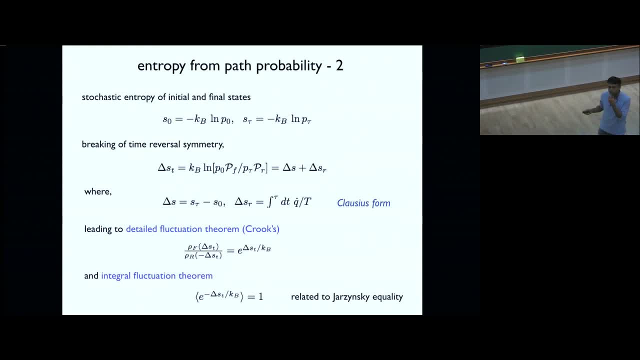 one can show that the total entry production in the forward path delta st, that probability of that and the ratio of the minus delta st. they obey this detailed fluctuation theorem structure And of course it's related to the integral fluctuation theorem. 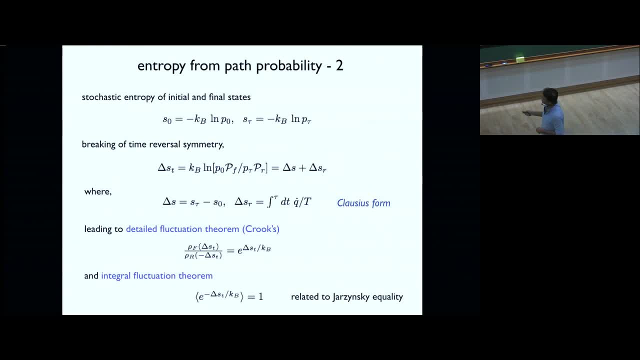 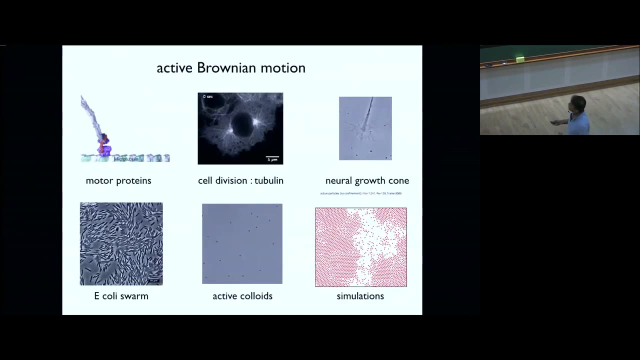 which is again related to Jarzynski equality etc. So these are the things we can get from single Brownian particle driven by external forces. Now I come to the active Brownian motion. So of course I don't have to motivate this active Brownian motion. 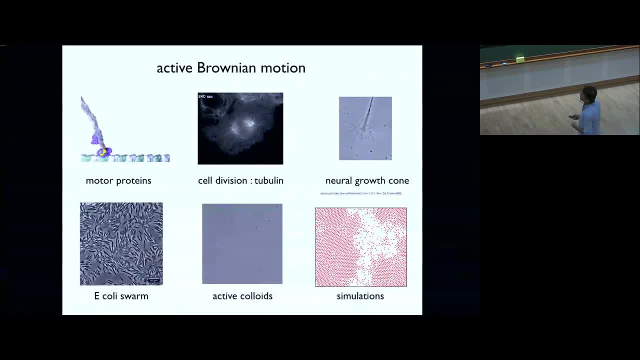 to this audience. We get to see activity in various biological situations, for instance motor proteins, E coli motion, cell division, active colloids and maybe neural growth cone motion. So some simulation of active colloids, So many such things in which the main issue is that 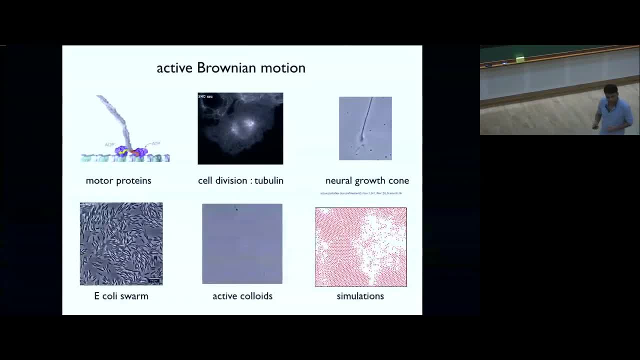 individual particles, as the conference website also says, that individual particles are self-driven, self-propelled, So they have some internal energy source. They use that. So the forces drive comes from the smallest scale, not from the largest scale. So that's activity. 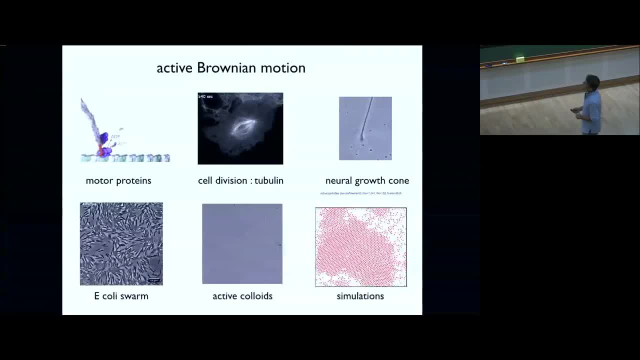 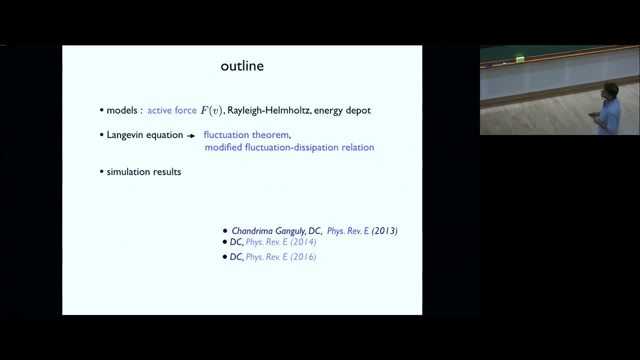 So then, my plan is to give a couple of models of activity which we will be using, some active force model, velocity dependent models, And then I'll give you outlines of fluctuation theorem and some modified fluctuation dissipation relation that's obeyed by the systems and some simulation results. 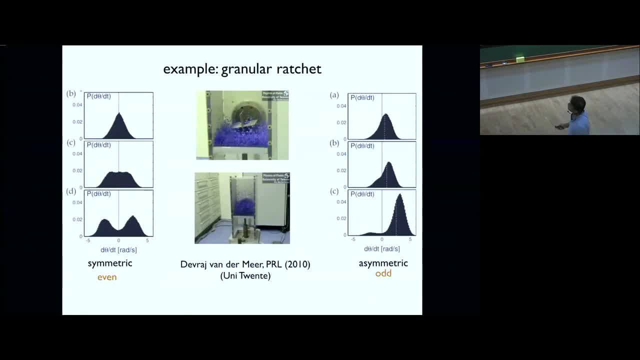 Okay, so before I get into the models, a little bit of motivation. why this specific model we are taking? So let's say these are experiment I've taken up from this reference. Let's say there is this fan which has blades. 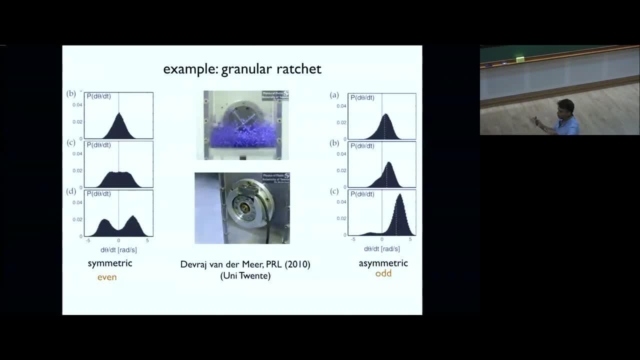 which are all symmetric in both sides, all the blades are symmetric in both sides. And then there is this kick from this granular material which is being vibrated vigorously, and they are kicking this whole thing And this moves either right or left. 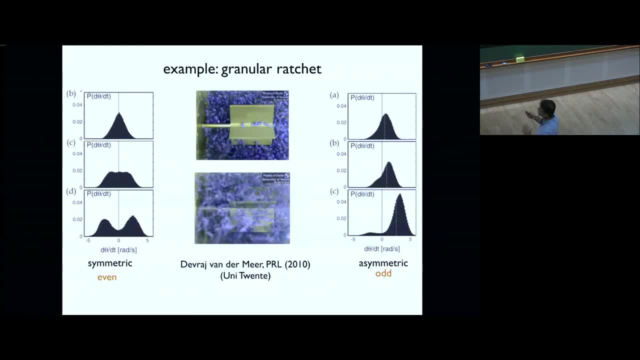 either clockwise or anticlockwise, So this thing being completely symmetric, if you look at the rotational velocity distribution, you'll see that as you increase the kicking of the whole stuff. of course the measurement depends on the time window over which one measures the velocity. 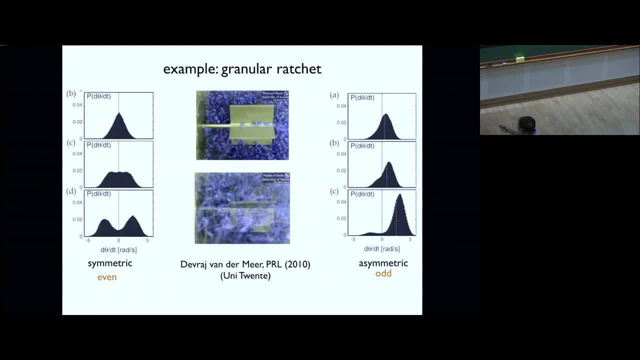 So, but over the time window, if you don't change the time window, you can see that the distribution of velocities picks up a sort of symmetric distribution where there is a positive and negative velocity. So maybe I can run it once more. You'll see that these guys make these blades move clockwise. 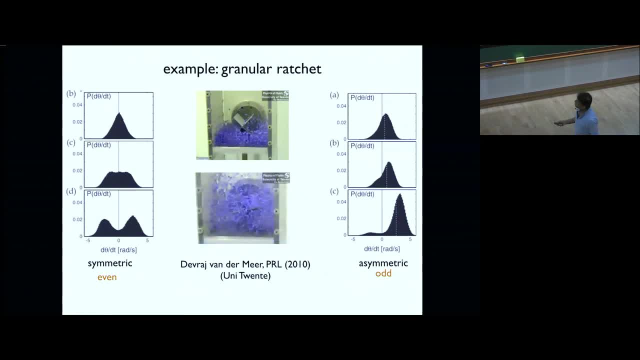 and anticlockwise, stochastically of course. And so this is weak driving. this is strong driving, in which it moves, or some period it moves in one direction, some other period it moves in the other direction. Okay, so I think this is a movie of the asymmetric bend. 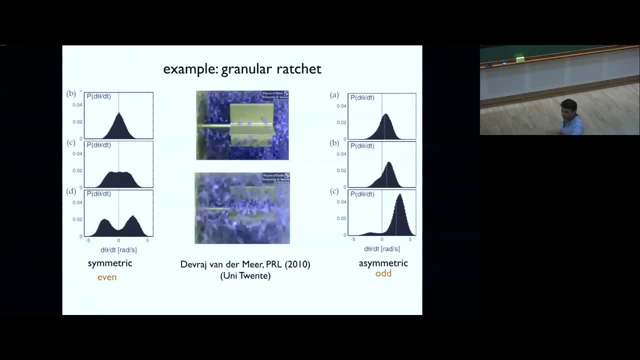 So one set of experiments were done where each blade is symmetric in both sides. Another set of experiment is done where one side is different from the other side. So this asymmetric thing then rotates in a specific direction and then you will get a velocity distribution which also picks up a little bit of negative peak. 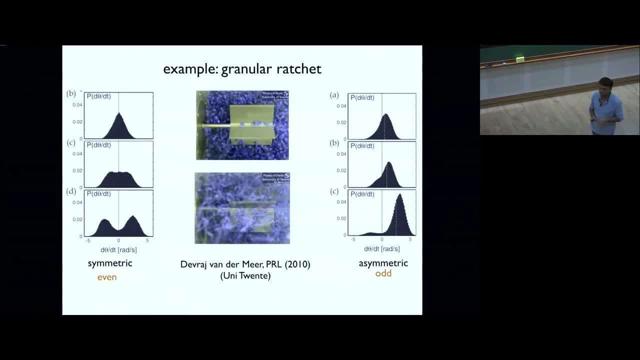 but mainly it remains positive. So what I'm trying to show is that the velocity distribution in this system, the effective system, which is rotating, that velocity distribution could be both symmetric, could be asymmetric. that depends on the system itself. If you make the system symmetric, it's symmetric. 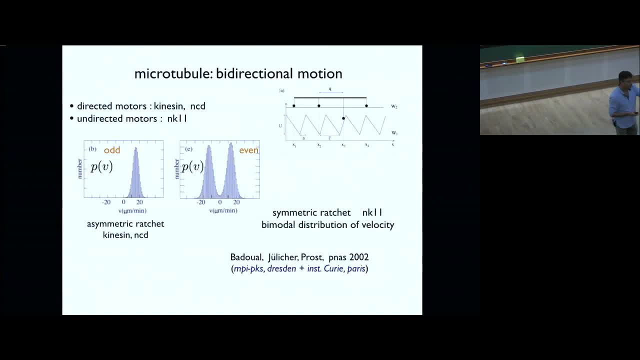 Then there is this: two surfaces of the blades. So I don't really remember now exactly how, how the asymmetry is generated, but this asymmetric in the way that if it rotates in one, rotating in one direction is favorable than rotating in the other direction. 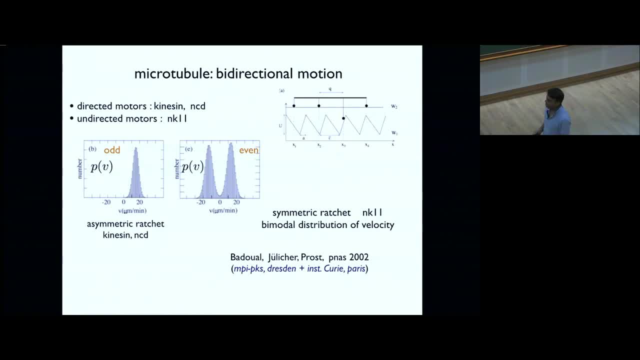 then you are kicking the whole stuff. So the next set of motivation comes from this: old experiments and theoretical explanation of the experiment. So this was. this is the experiment about a microtubule being driven by kinesing like molecular motors. 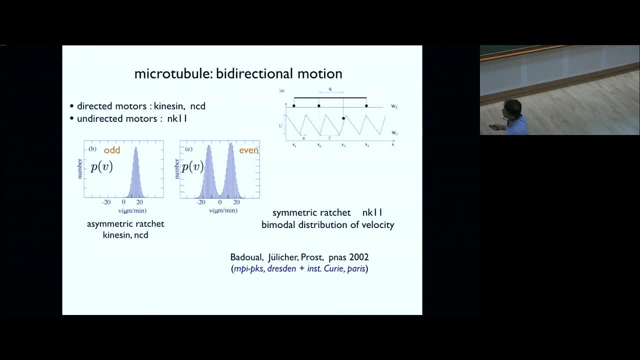 One kind is this: normal NCD motors, which will take the microtubule in a specific direction. Each individual motor moves in a specific direction and many of them are carrying this microtubule, So the microtubule is as a whole. 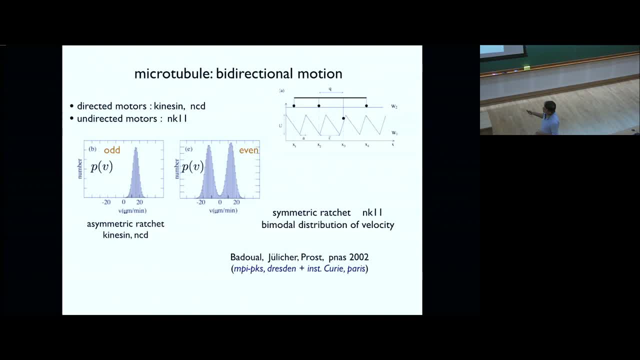 carried in a specific direction. And if you look at the velocity distribution of that that guy- so sort of how many times it's going forward and how many times it's going it's going backward- So if you look at that, that guy will show a positive motion. 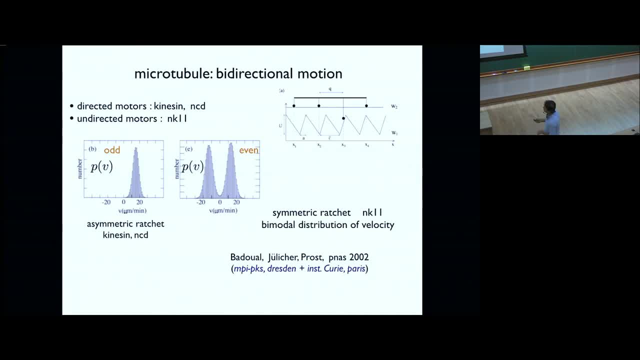 positive velocity in a specific direction. So that depends on the orientation on the microtubule. On the other hand, there was this other protein which belongs to the same kinesing family, NK11.. So this guy is behaves like a symmetric ratchet. 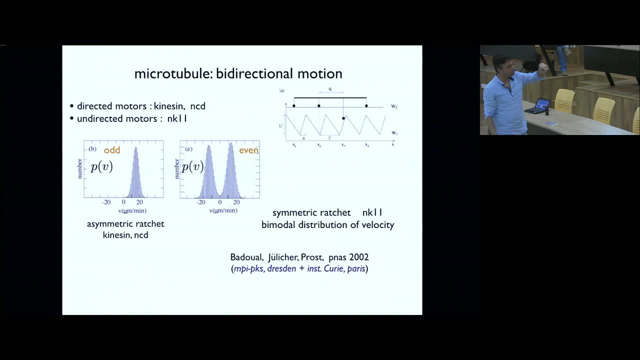 in which essentially the microtubule undergoes a symmetric motion. So it shows you some one period it shows a positive velocity, other period it shows a negative velocity. So you have to imagine that single microtubule being driven by many of these motors together. 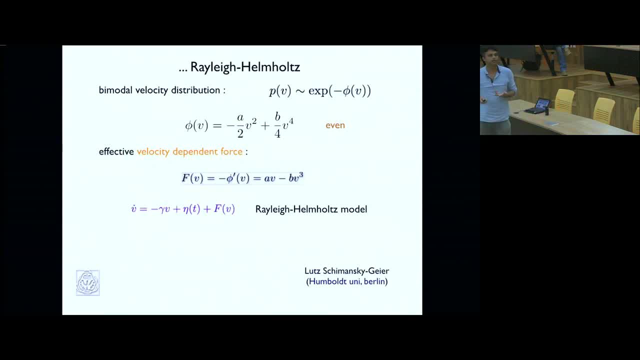 And then the symmetric case. obviously, this distribution looks like a symmetric distribution which can be captured by velocity dependent potential, and the velocity dependent potential then can be used to write down a velocity dependent force which was being written for that specific case and certain experimental results. 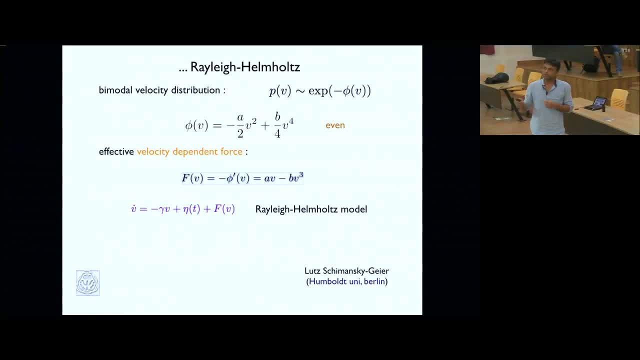 could be analyzed using these equations. So but if I write down this equation, or equation of motion in presence of such a velocity dependent force, this is called the Rayleigh-Helmholtz Model And this model. so main thing we should focus on, 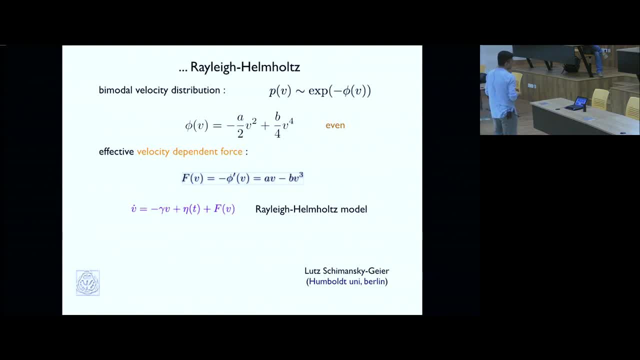 is that this velocity is the force itself is odd in the velocity variable. So if I take velocity, velocity is equal to the velocity variable t. going to minus t, velocity will pick up a negative sign and these forces will pick up a negative sign. So this is unlike the external force, It picks up a sign under time. 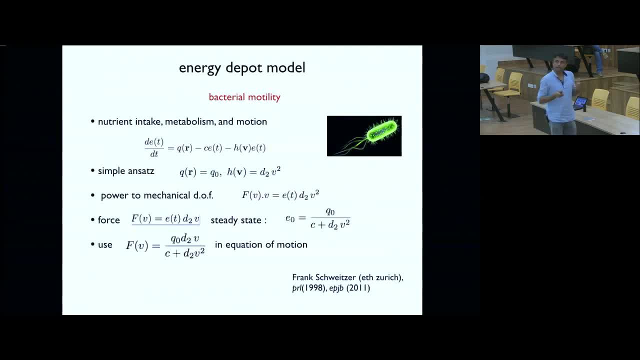 reversal. So then there is another class of models. It's called energy depot model. So this like to describe a naive description of motion of a self-propelled particle. So what you can do is that we can say that the particle is moving because of an internal 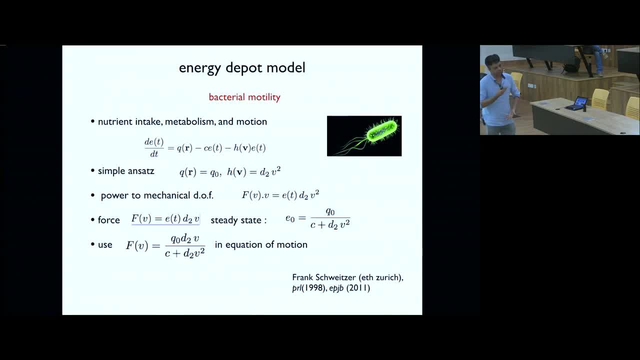 energy depot. and the energy depot has dynamics of itself and part of the energy is supplied to the motion of the system. So what could be the naive dynamics of such internal energy depot? That, let's say I'm thinking about a bacteria. The bacteria eats some food, so 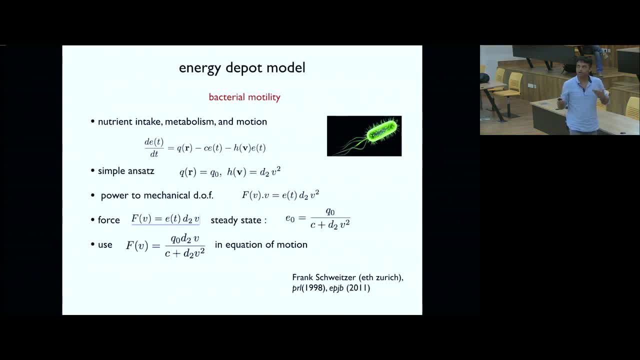 that's an energy increase, the gain term, Then it has to metabolize, so part of the energy will be lost to metabolism And then there will be a part of the energy that is which will be utilized for motion of the bacteria. So if I use that part of energy, 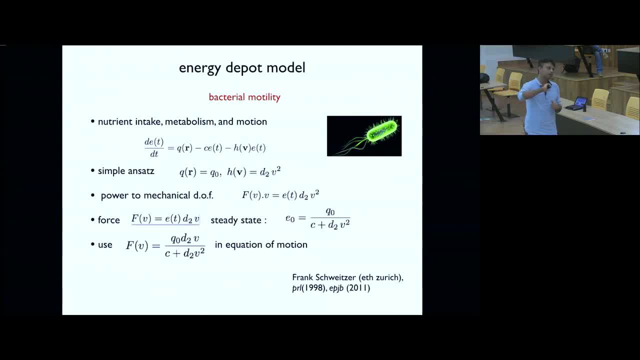 so simplest would be if the bacteria doesn't have forward-backward symmetry breaking. if going forward, going backward is equivalent for the bacteria, then we can imagine that the energy lost to motion should be to smallest order, should go as v-square. 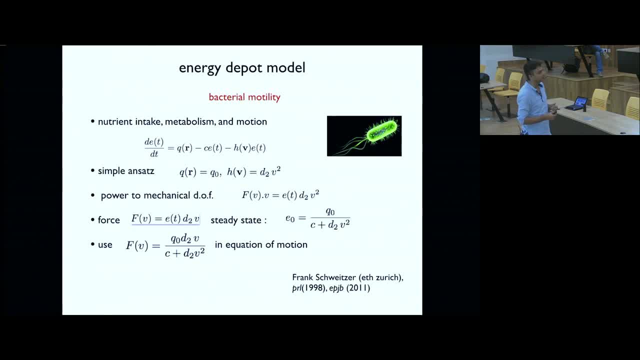 So it should be symmetric under v-positive and v-negative. So it doesn't matter whether the bacteria moves towards right or towards left, It has to use up energy. So that part of energy, if I then write it down, so this is like an energy dissipation. 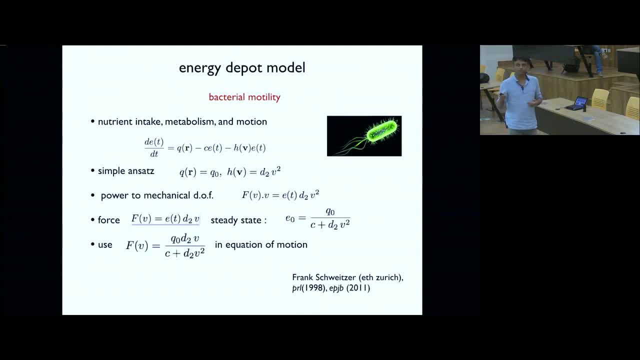 which is like a force times a velocity, And this force will go to the motion making of the bacteria And that force- then I can use this relation- that force will be then given by instantaneous energy of the bacteria: E-T times this velocity. 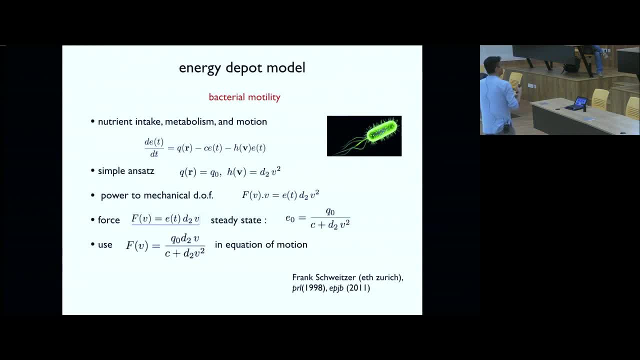 But we can use a simplification, say that the bacterial internal energy depot equilibrates faster, So the dynamics is much faster, not equilibrated. It goes to a steady state faster And if it goes to a steady state one can use a steady state assumption. 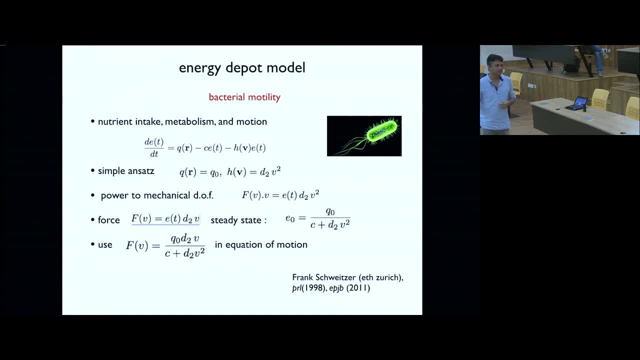 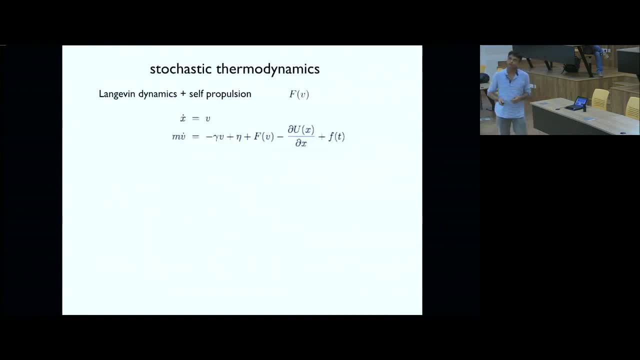 And then you'll get a steady state energy which is even in velocity, And as a whole you'll get a force which is again odd in velocity. So with this motivation, now in the first part, let me show that what will happen if I just use velocity-dependent forces. 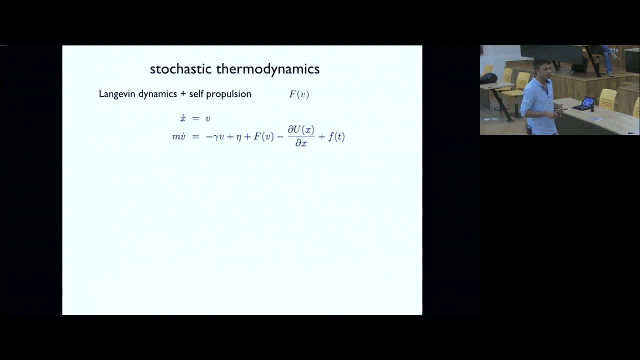 where the force is odd under velocity, so under time reversal as well. So first thing is simple. So if I try to look at energy conservation, I'll get an energy conservation. So this part and the potential energy together will make the total energy. 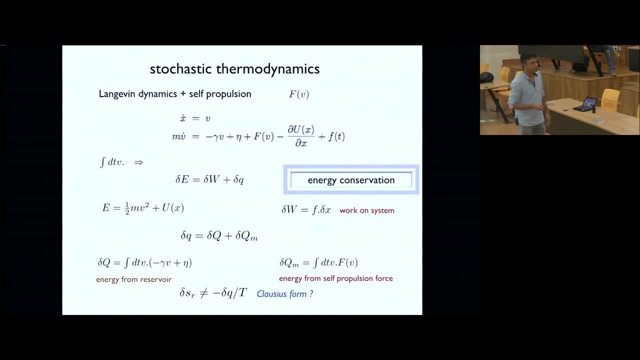 And then there is a work done. Work done is just external force, times, displacement for the bacteria, And then I'm left with two pieces. One piece is my original energy from the reservoir, So that's the heat. And there is an extra piece. 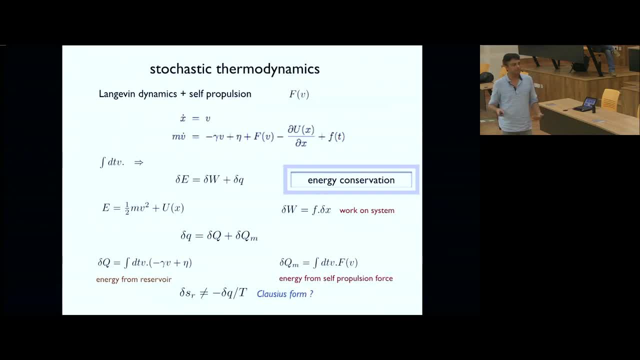 which is some kind of a force times velocity, where the force is coming from the internal energy depot. So we can also at this stage interpret this as another reservoir which is internal to it and that reservoir is supplying this amount of energy. 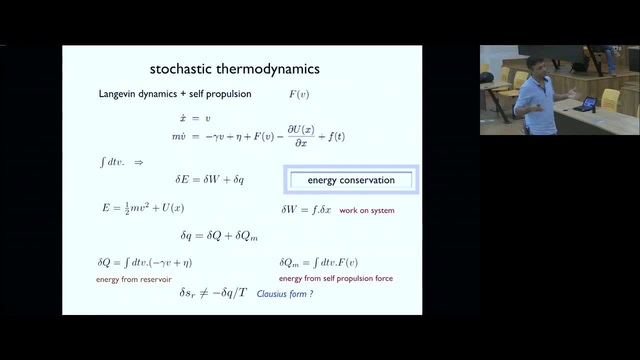 So then you'd expect that from here. if everything was fine, I should have got a total entry production in the reservoir, which is just addition of these two terms. So what we see is that the unexpected part is that this doesn't hold. 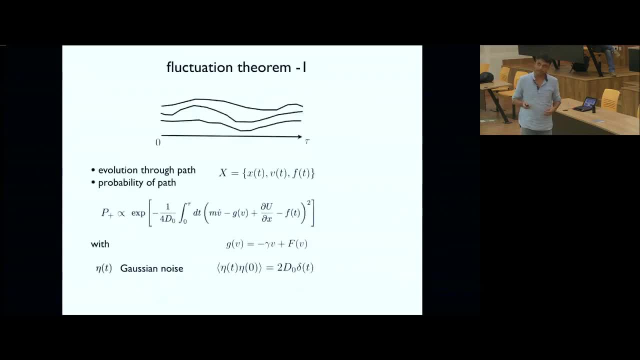 So we have some extra bit on it. So we just use. so we use our normal. so we can either use Fokker-Planck equation or the time forward time reverse trajectories to calculate the entry production. So same algorithm if you use 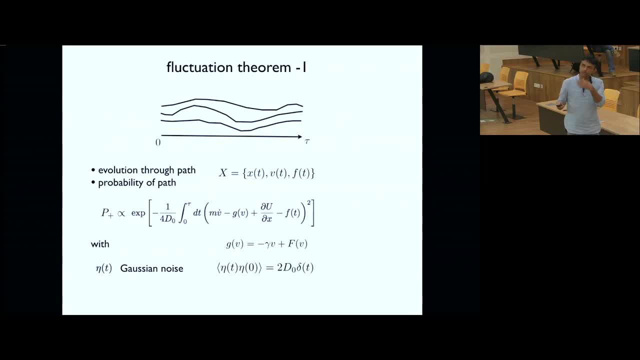 so of course there will be a Jacobian sitting here, but in this specific case the Jacobian drops out under time forward and time reverse probabilities. So if I take that ratio, so in the ratio what comes out is that, apart from the total heat absorbed, 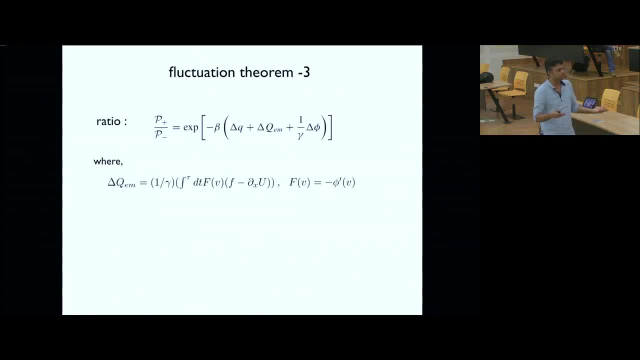 by the system, from the reservoir and from the internal energy in the mechanical degrees of freedom. apart from that, there are these two extra bits And these two extra bits. so first bit you can look at. so this is given by a cross. 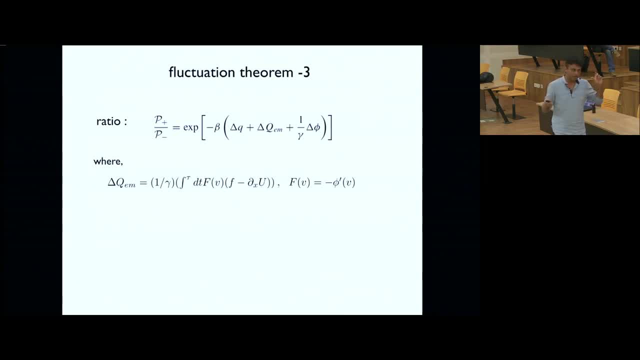 this is a cross term between the force production due to the internal energy bath and all mechanical forces, external force or potential, etc. This is a cross term between the two And the last part, this delta phi, is coming from the velocity generation. 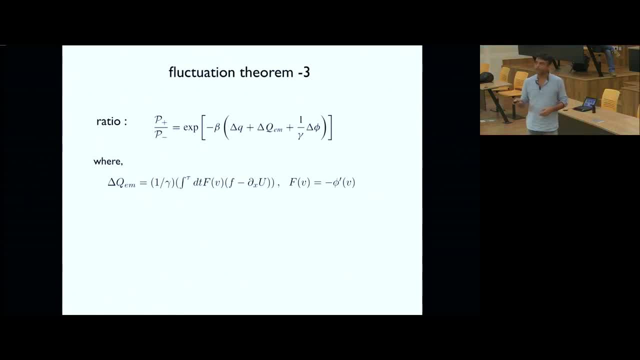 by the activity of the bacteria. So this is just minus del phi del v. So with respect to velocity it acts like a potential. So and then you can do the regular stuff and show that the entire production in the reservoir has this extra part, extra bit. 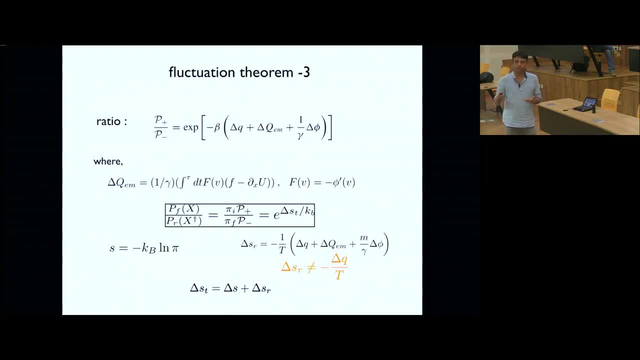 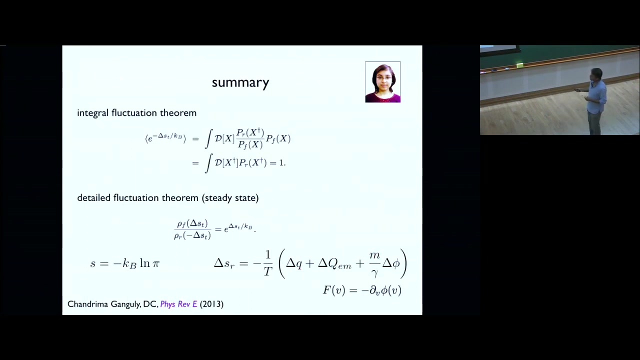 And of course this whole thing obeys fluctuation theorem. But this extra bit is really coming from the crosstalk between the internal energy bath and the mechanical degrees of freedom. Everything else follows the integral fluctuation theorem. detailed fluctuation theorem At steady state. we are now thinking about a specific steady state. 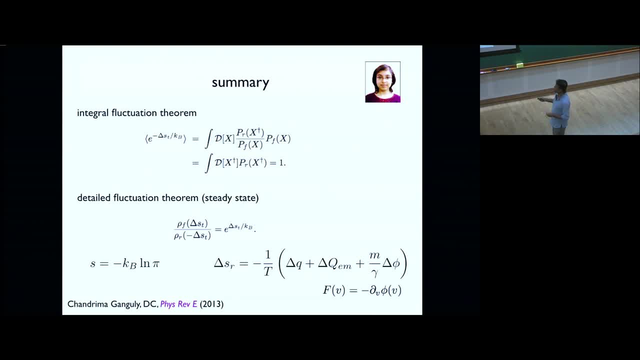 under constant drive And then you have this total entry production which has this extra bit. So this extra bit is the thing which is the main. I'll say new result and we don't understand exactly. So understand in the sense that if I try to interpret it in terms of really two baths, 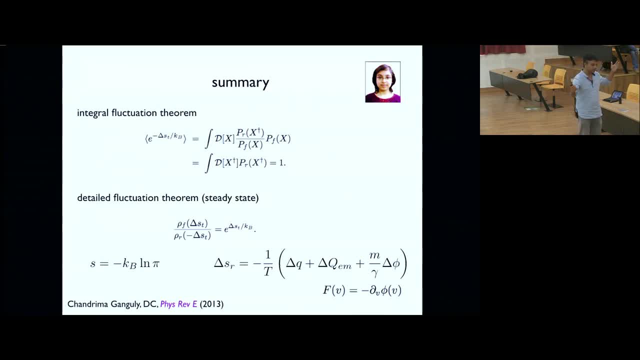 so I would have liked to see something where there are really heat dissipation in the baths to begin with. So maybe I start with something like an equilibrium bath And then if I come to a non-equilibrium counterpart of it, then we should see where from these extra terms are coming. 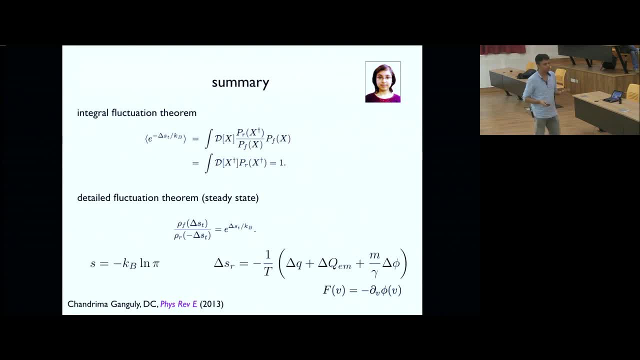 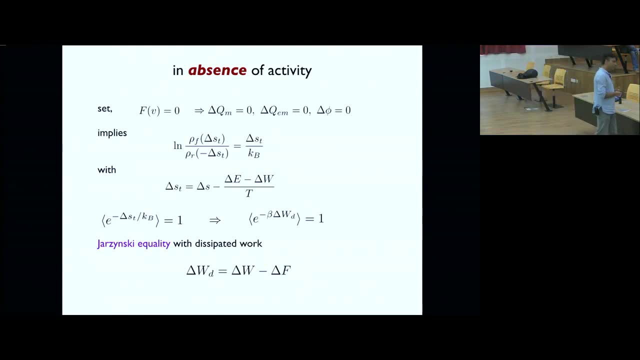 So we can see within this calculation where from they are coming, But that's just within the specific models. So models which are given by this velocity-dependent forces which are time reversal asymmetric. So of course, if you switch off these velocity-dependent forces, as I assured that we'll get back, 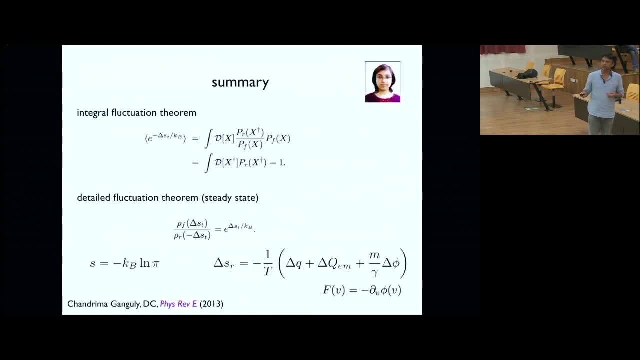 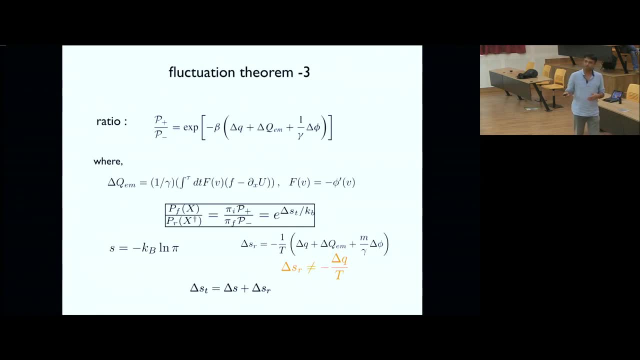 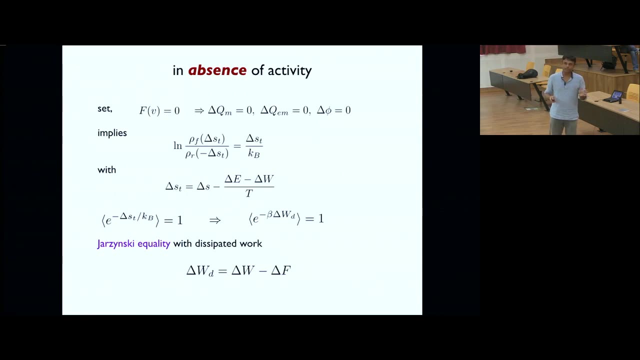 this delta Qm. So the moment I switch off velocity-dependent forces, all these extra terms drop out, Because everything has this bit of Fv. So they drop out and we get back our original Clausius form of reservoir entry production. And then of course it obeys Jarzynski equality, etc. 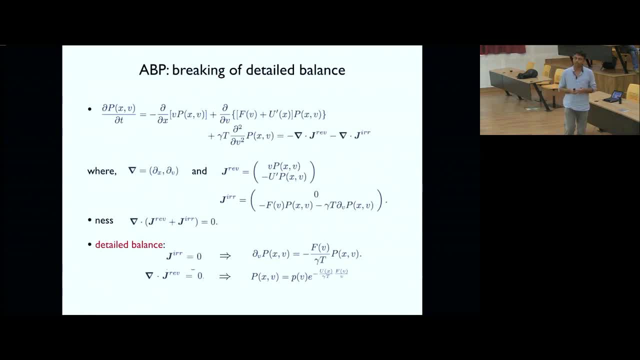 So then, if I come to our system and ask this question, that what is the minimal condition under which the system shows breaking of detailed balance? So I wrote down the full Fokker-Planck equation of this system, My reserve, reversible and irreversible parts of current. 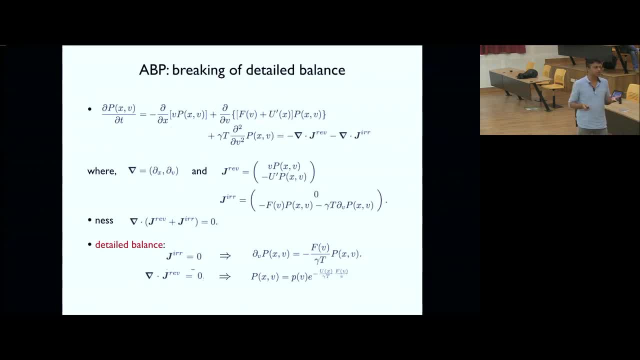 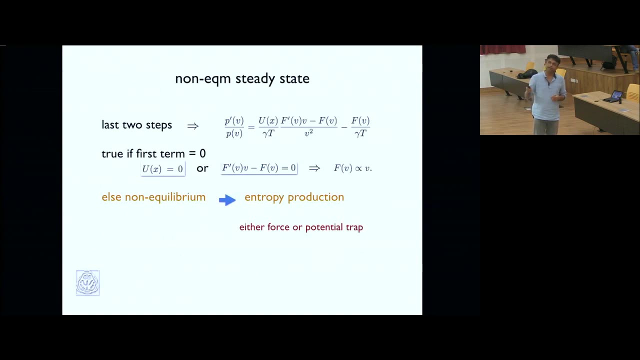 I list down here. And the detailed balance condition will require that irreversible current is zero, while the divergence of reversible current is zero. So you have these two equations Now, if I put these two equations together, I get this relation. So this relation is something where I have in the left hand side. 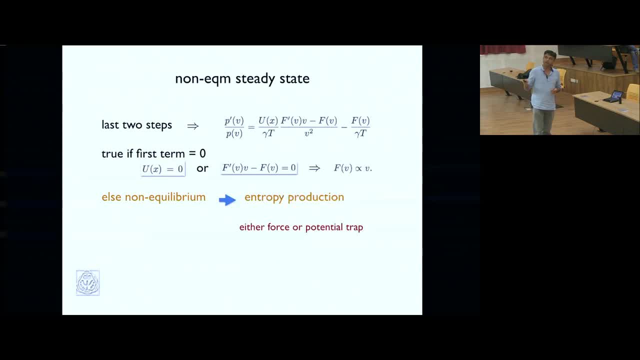 everything is a function of velocity On the right hand side. this guy is only a function of velocity, But this guy is sitting here with a function of position as well. So this cannot be true unless I set ux equal to zero. That's one possibility. 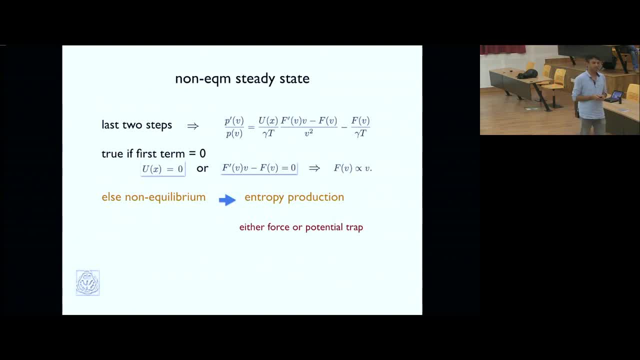 Or if I set this Fv is proportional to velocity itself. So that's like putting this time using only minus gamma v as the velocity term. So that's like equilibrium bath. I'm at equilibrium, Else I have to set ux equal to zero. 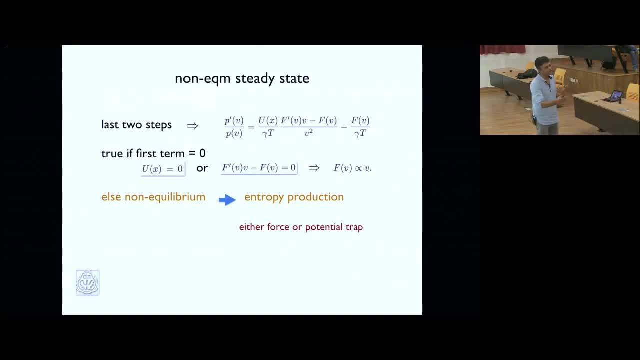 then the system will behave like in equilibrium. So detailed balance will be obeyed and one can also write down the probability distribution, which will have a different structure but obeys detailed balance. So it shows us a possibility that even if I take this particle and put it in a harmonic potential, 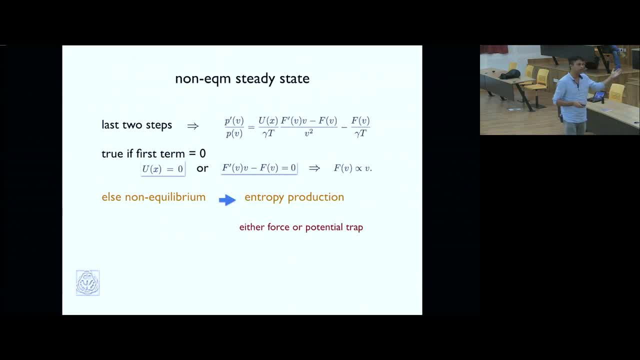 it will start to produce entropy, So I don't have to really use external drive to produce entropy and drive the system out of equilibrium. So the system will go to non-equilibrium But by itself free system is still obeying detailed balance. in this case, 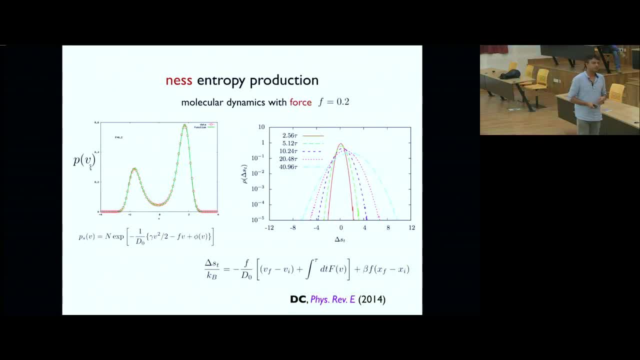 So first thing, simpler thing: if I put just an external force, the system produces entropy. So this is the probability distribution of the velocity And the entropy production. this is the distribution of entropy production. So I just wrote down the expression of the entropy which we used. 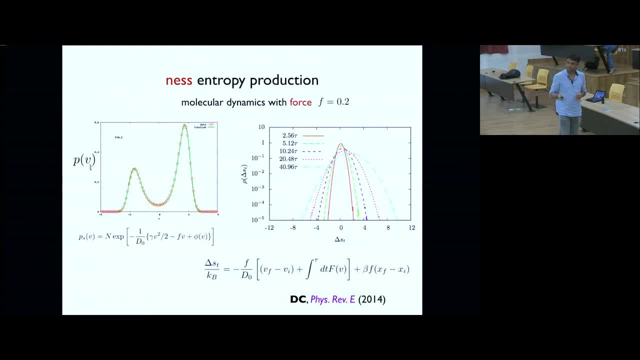 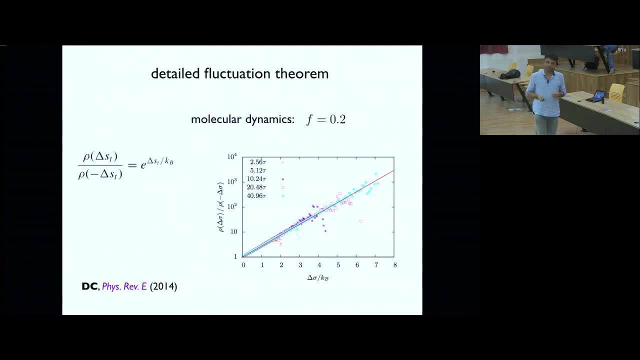 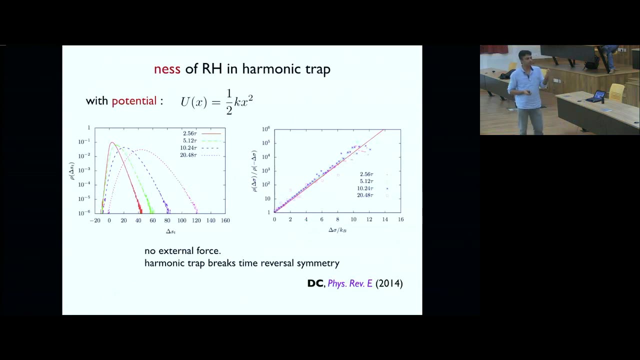 to do this calculation. This is the calculation numerically, And if I take those probabilities, they obey the detailed fluctuation theorem nicely. The second thing is, if I put this particle under external trap, just a harmonic trap, it's again driven out of equilibrium. 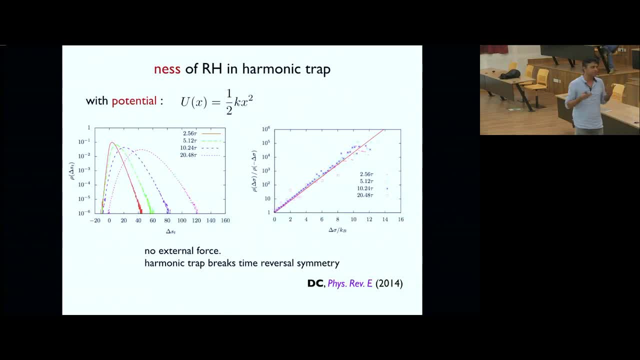 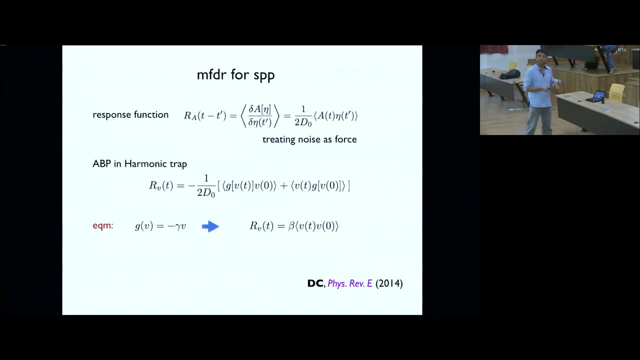 and it produces entropy by itself. So it starts to behave like a self-propelled particle. And then these are the entropy production, the probability distribution of entropy production, and again it obeys the fluctuation theorem, symmetry. So for this system, then the next question I come to. 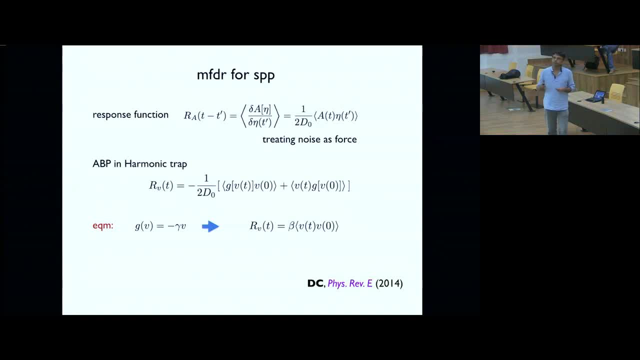 this fluctuation-distribution relation. So the response function one can calculate by using the noise in the system, treating it as equivalent to the external forces, and then we get this relation where noise is involved and then we can use our equation of motion. 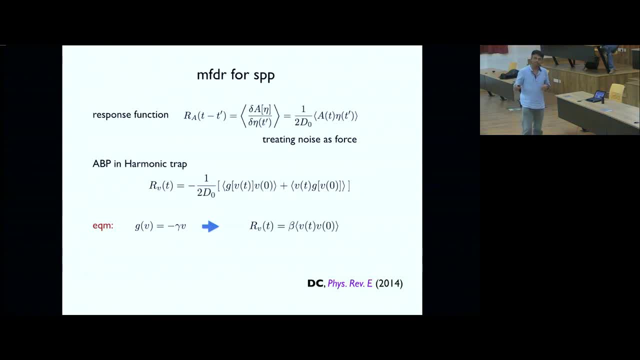 And using those, so some steps of algebra, one can show that the velocity response of this system, in presence of this external harmonic trap that has this structure, where I have a correlation of this G, G is taking care of all the time reversal. 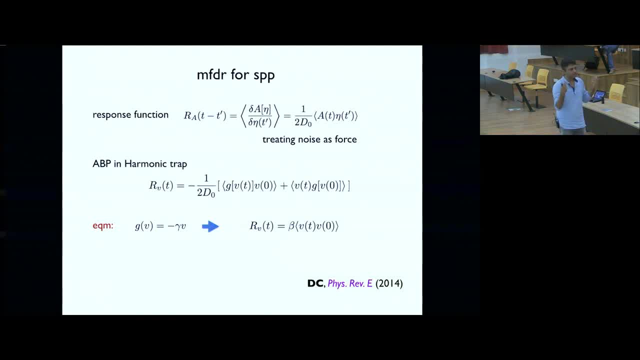 asymmetric velocity-dependent parts like minus gamma V and the external force F of V. These two together I'm calling that G, So this guy. of course, if you are driving it out of equilibrium, this correlation is not equal to that correlation And that one can also show explicitly. 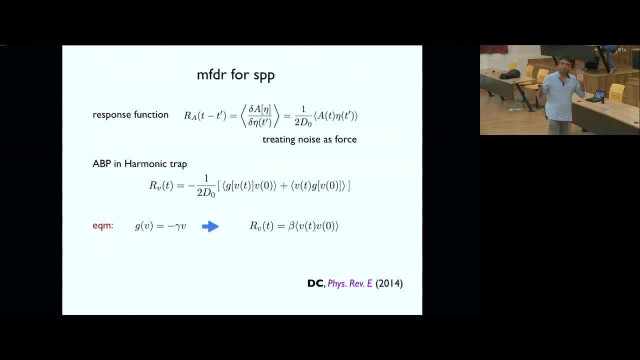 And one can separately calculate it. So what the next thing I'll show is that we can separately calculate this correlation and that correlation at a steady state for active Brownian particle in a harmonic trap separately, And then we drive it and look at the response. 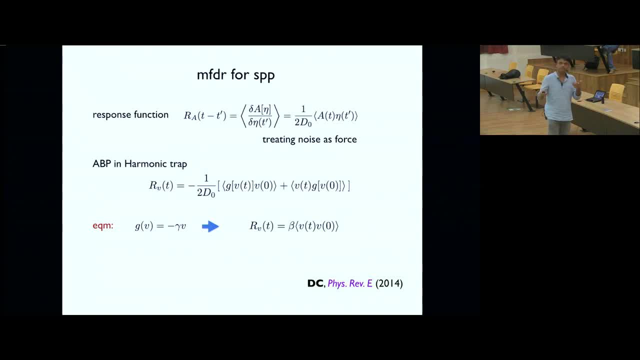 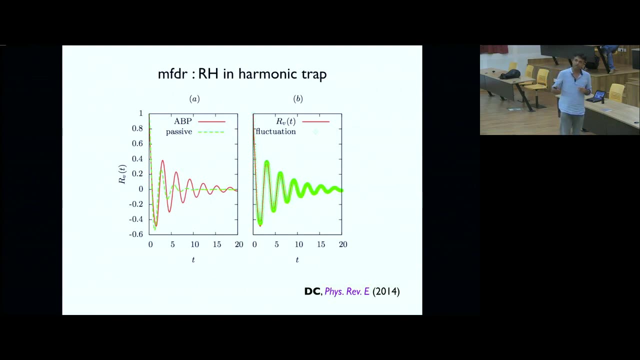 and compare these two. And of course, if I just put GV equal to minus gamma V, I trivially get back the equilibrium fluctuation distribution theorem. So this is the response. So what I'm showing in the first graph is the response function. 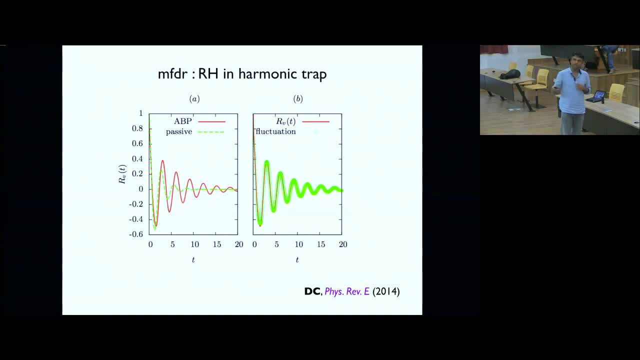 within this harmonic trap for the passive particle and for the active Brownian particle. So active Brownian particle shows much longer correlation and longer time of oscillation. And then here I'm showing the comparison between the fluctuations: steady state fluctuations with the response under small external kick. 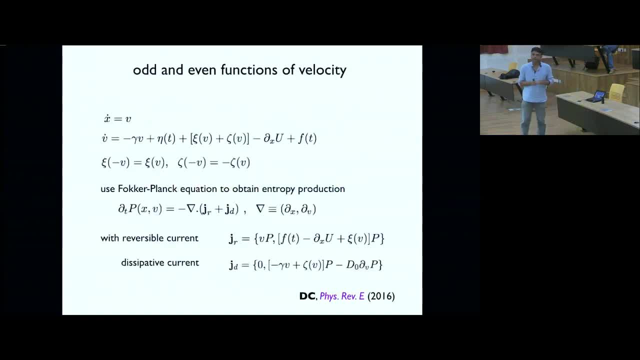 So they match well. So then I come to our next generalization of the model. So this part. earlier I said the external velocity dependent force. what I'm introducing is asymmetric under so is odd function of velocity. So now, if I use both bit, 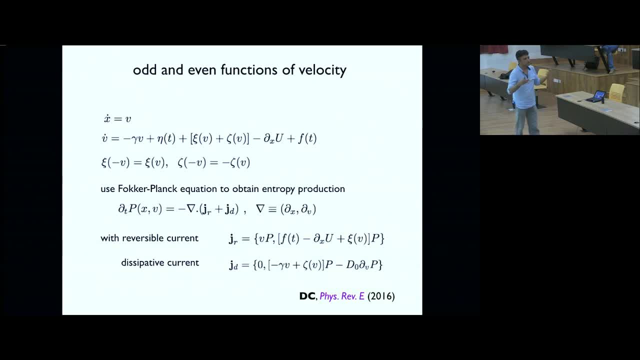 one is an odd bit and an even bit. So I assume that the velocity dependent external forces can have both odd function of velocity and even function of velocity And if I can separate them out. So one is even and another is odd, And then I go through the same steps. 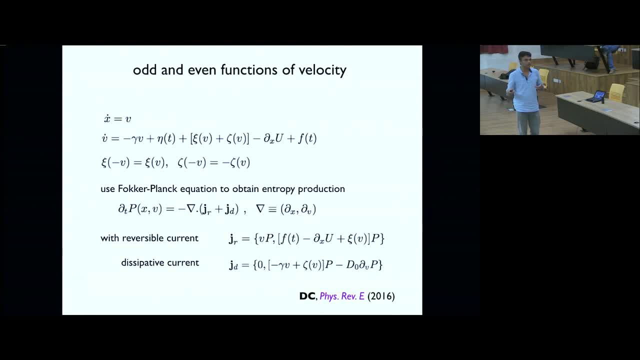 you'll see that the reversible part- now reversible part- of the current will have this odd function of velocity sitting here. Sorry, the even function of velocity sitting here, And the odd part, like the minus gamma v, goes in the dissipative part of the current. 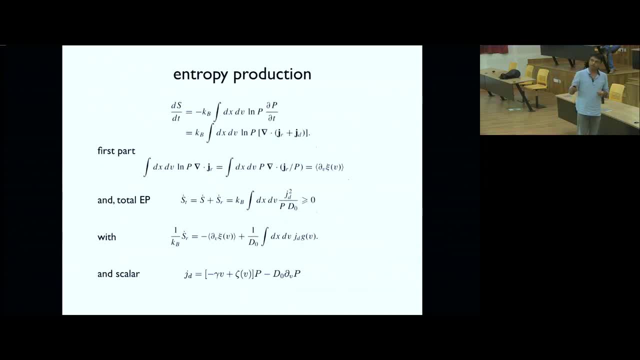 Strangely, as you'll see that, if I now use this entry production, so we have again used the Fokker-Planck route and the time forward time reverse path route to calculate the entry production in the reservoir. So I'm just showing the Fokker-Planck route. 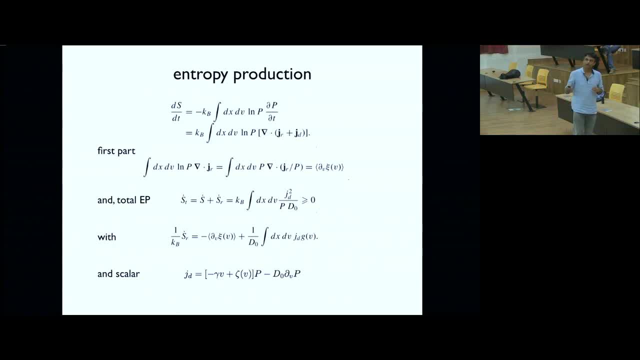 Both these results match with each other. I'm showing the Fokker-Planck route, and so first part, the reversible part, as I showed earlier, will have a p times divergence of jr by p part, which now for this specific case. 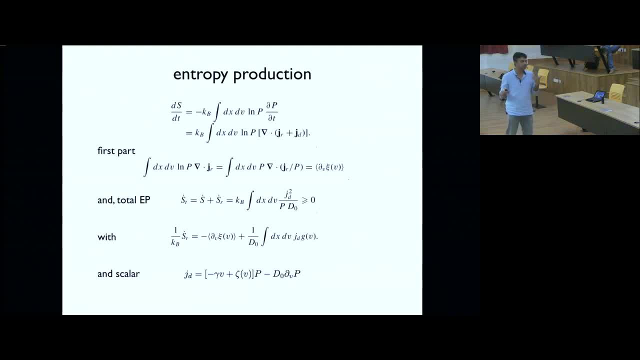 is not zero. So this velocity, derivative of this even function of velocity, the active force, which is the even function of velocity, And then in the total entry production, I have this part and extra part which is the dissipative part of the current. 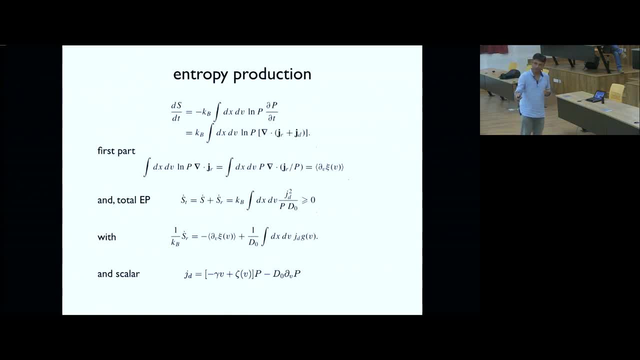 So I just look at the total dissipative part of the current and pick out this bit. So this bit of the dissipative part of the current, the other bit is zero. So I just pick up this and I'm calling the scalar dissipative part. 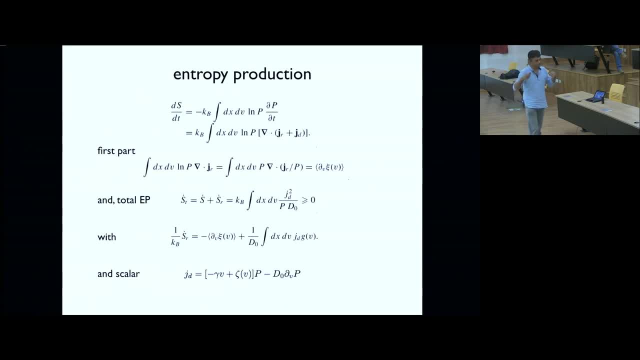 of the current and that scalar current and the g of v, which contains all the odd velocity dependent terms minus gamma of v and the odd part of the velocity dependent forces that together. So if I take them so that together ultimately generates the total entry production. 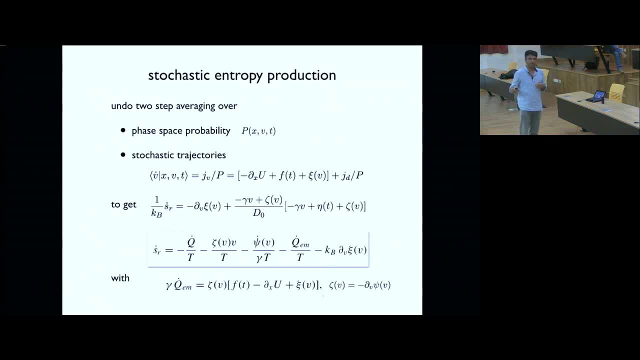 in the reservoir, So in the total entry production in the reservoir, apart from the heat dissipated, heat absorbed from the environment, then there is energy produced by the internal energy depot. that comes to the energy flux, so that two of them are in this q dot. 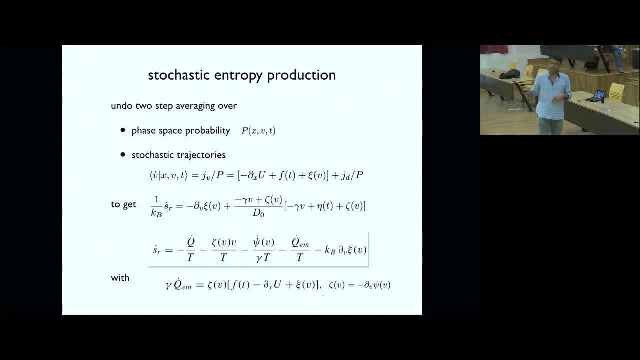 and apart from that, we have this all extra terms and in this expression. remember that I'm not using the external force anymore in this expression. Even if I don't have external force, I'll still have all this because I have the odd part of the velocity. 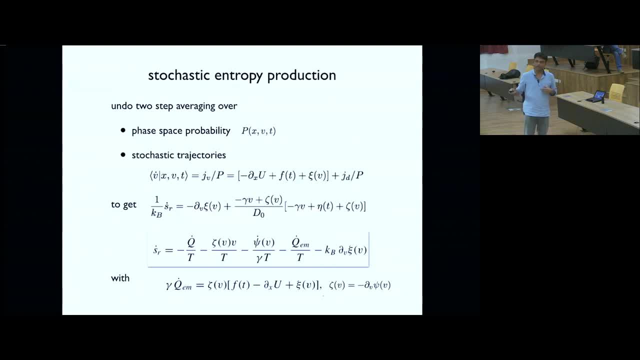 and the even part of the velocity they are coupling together. And these guys together are the, all of them together constitute the non Clausius dissipations in reservoir, The reservoirs I cannot point out now So because these are all coupled between, so these are coupling. 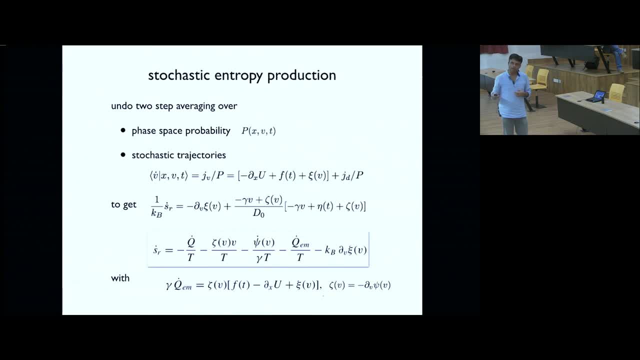 between the odd odd. this guy's psi is given by the, so this is the velocity dependent potential which will give rise to the odd part of the velocity dependent force. Then this qem dot contains the odd part, coupling with the even part. even if I have 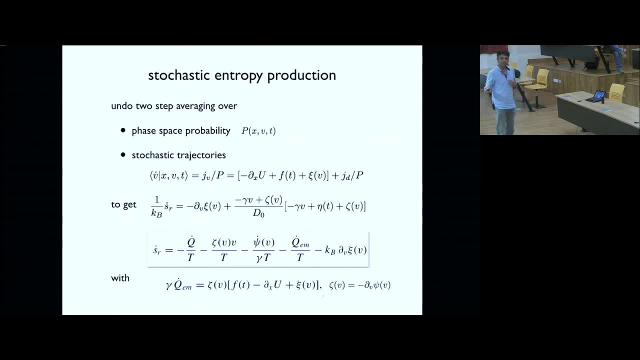 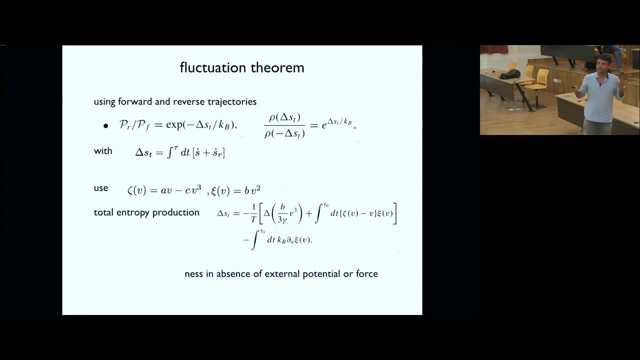 don't have external force or external potential, these extra bits will come in. So, but rest of the things follow, like the total entry production. if I use this entry production in the reservoir, that obeys this fluctuation relation, symmetry, and the total entry production has this: 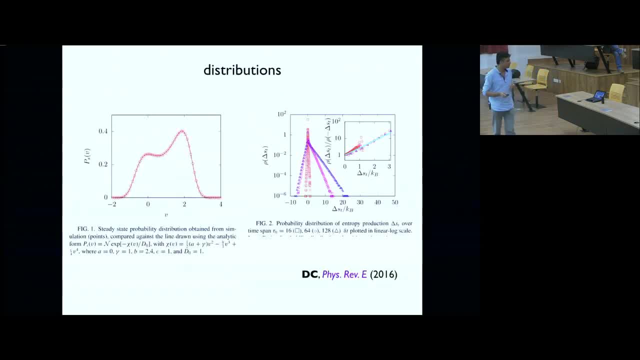 strange structure. then what I can do is that you can do a simple thing, that I can simulate this. So I take a particle in which I use this external velocity dependent, so I'm saying that this particle is driven by the velocity dependent forces and this velocity dependent forces. 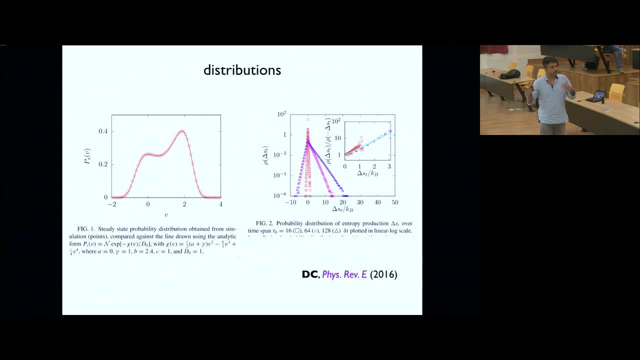 has in general, can have both odd and even parts. so one part is like the odd part, which is velocity dependent potential, will generate these even functions. so these are this v squared and v four terms, and another could be a v cubed term which will give rise. 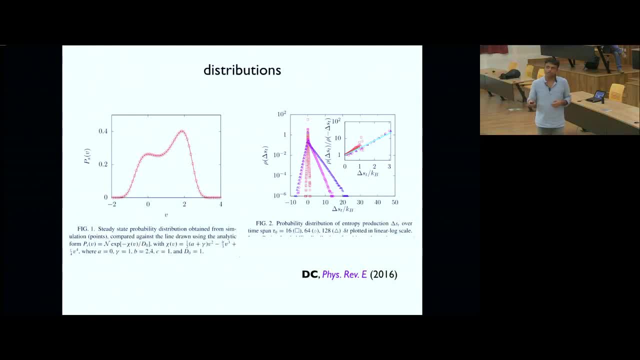 to a force which is v squared or even part of the force. So if I take them together I can write down the probability distribution and that matches well with the simulation results for the probability distribution of the velocity, and then I use this simulation to calculate the entry production. 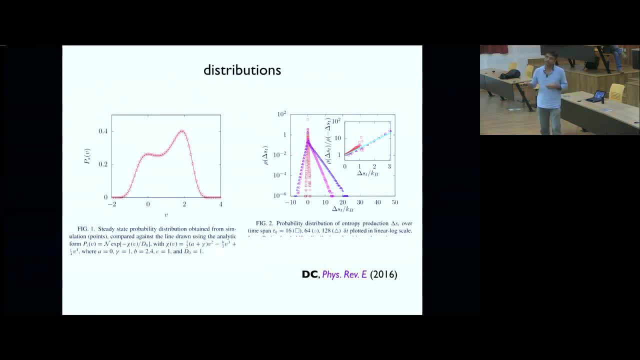 in the system, the entry production has this shape, but, but what still? it obeys the fluctuation, detailed fluctuation theorem, this symmetry quite well, and of course we don't. for this system we don't require any external potential trap or external forces to drive the system. 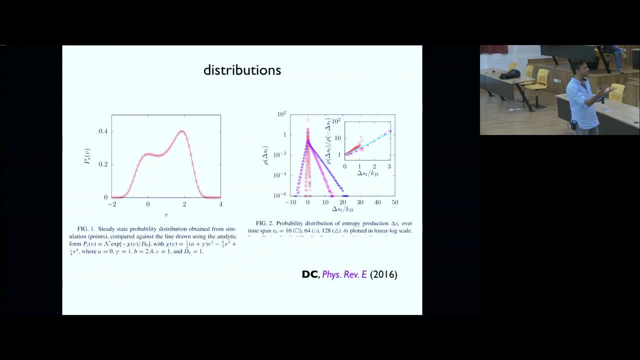 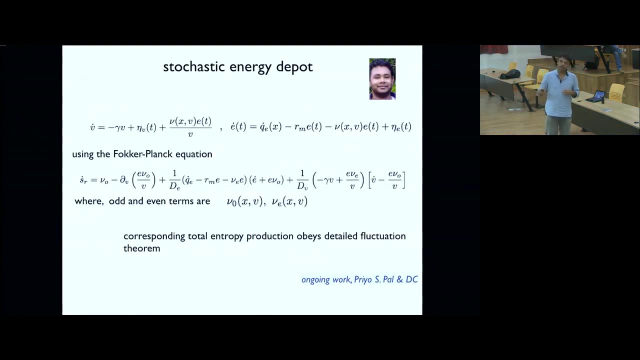 out of equilibrium. the moment I have both odd and even function of velocity as the velocity dependent forces generated from internal, but they will drive the system out of equilibrium. So, then, the last thing, what we are doing right now, is that if we write down a full stochastic, 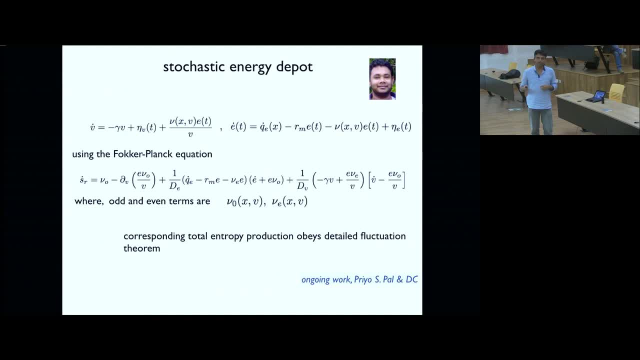 version of the energy depot model. so keeping a heat bath term. so we have particle moving in presence of this heat bath and where this guy is coming, due to the coupling with the internal energy depot and the internal energy depot. so we have the gain term. these two 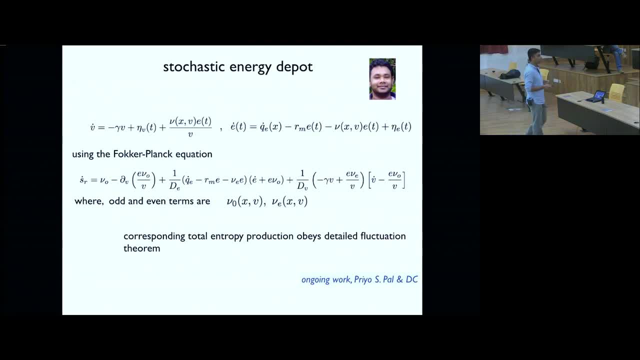 loss terms and the stochastic stochastic energy term in this. and then you can follow the Fokker-Planck route or the time-power time-reverse path route and try to calculate the entropy production in the reservoir. so again, the total entropy production, we can write. 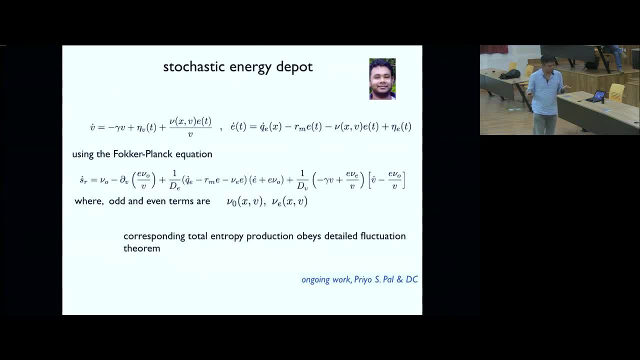 down as something which can be both odd or even function of velocity. so some terms are odd, I am writing them new- odd and some terms are even. and then of course I have not separated out the heat production in the reservoir here, but you can see that this bit 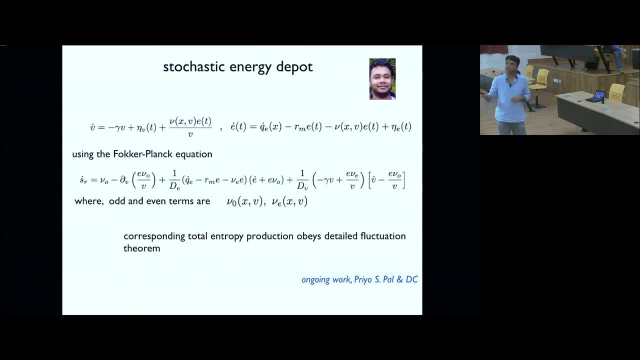 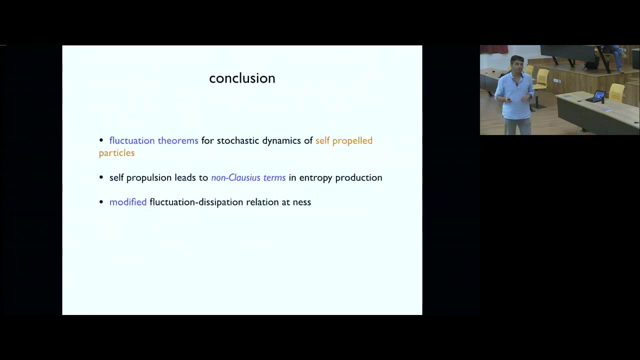 has reservoir force generation and that can multiply with this minus gamma V to generate the original heat production term. but there are many more extra terms coming just due to the forces generated from generated from the internal energy depot that gives rise to several non Clausius entropy production. 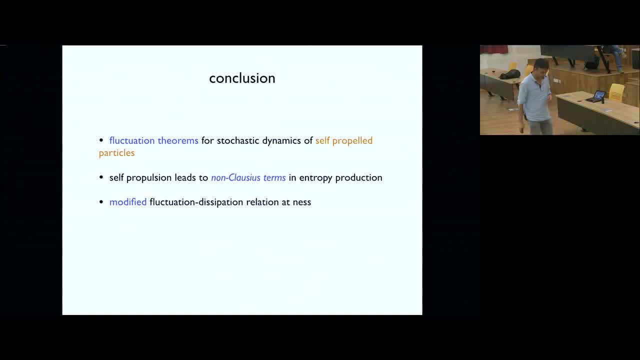 term, apart from the normal heat bath entropy production. so, and also we can see it in the state of mass in the atmosphere and in the atmosphere of the atmosphere. so this is the basic concept of the energy distribution and therefore the energy heat. so my, my suggestion would be to come up with a more microscopic model. 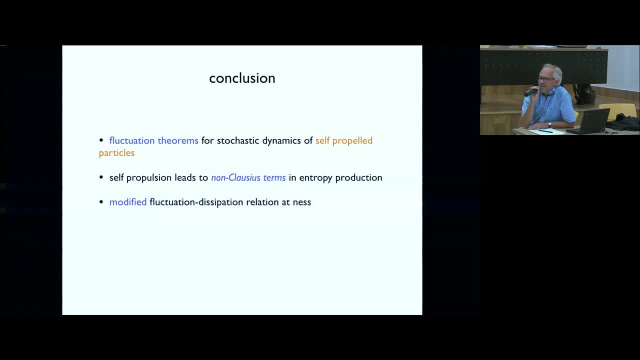 which mimics or reproduces this kind of f of V behavior. and then the whole issue of entropy production would be clear, because for the microscopic models it's pretty clear what physical entropy production is here. so I had been thinking in this line. one problem is with the energy depot kind of models is 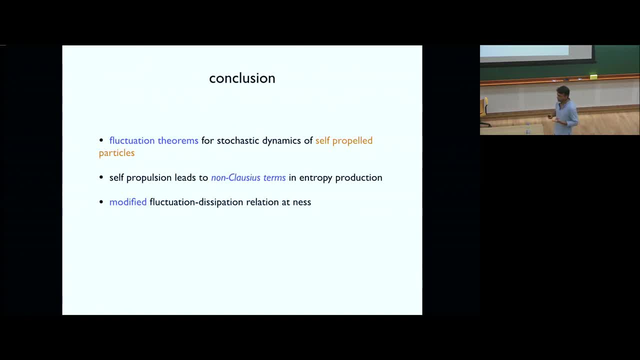 that the other equation is the equation on energy that's not in the same status. instead of that, probably one possible way could be- so I was thinking about it, then try it out. so one possibility could be that if one takes two beads connected with, let's say, a spring, and say that the first bead is coupled to the, so it's a. 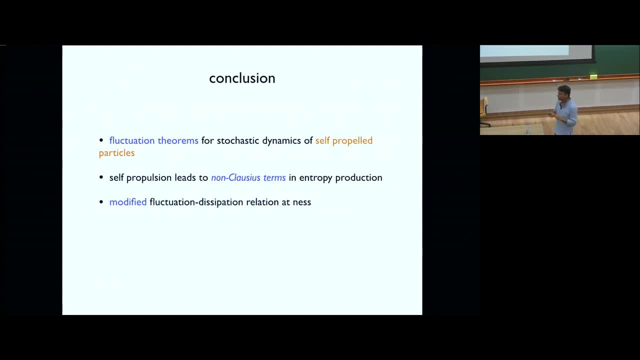 bigger bead which is connected to the first bead and the second bead is which is looking at the external world and there is something internal, so which can be mimicked by the second bead and it could be a different reservoir. for instance could be a correlated noise reservoir correlation often people use 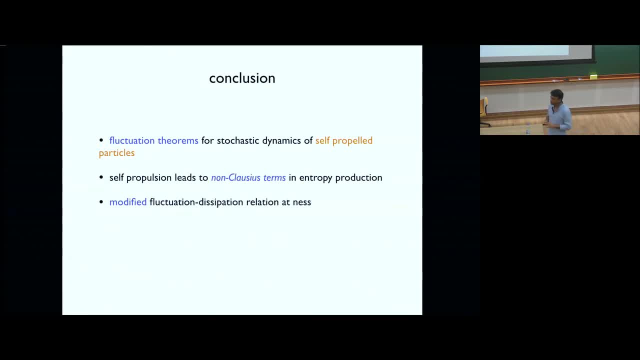 for modeling activity, and then one can try to separate out. so my, so in one thing I am getting convinced about the calculations. so that's the reason I'm also asking you this question: that entry production, we can write down, the introduction structural, the intro production from time for our time, reverse trajectories. that's one. another possibility is that 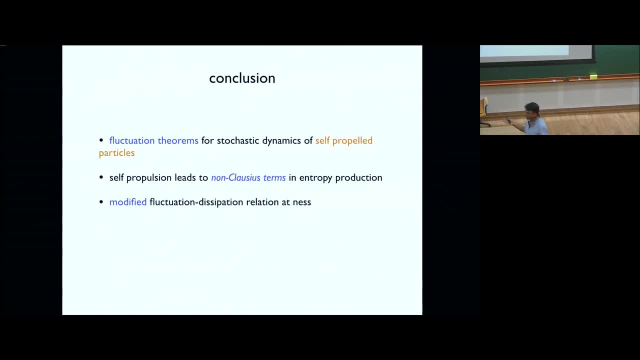 we can take the Fokker-Planck equation of the whole system and then try to identify what are the interruptions. but in both cases it for this kind of phenomenological models it will be more a kind of effective entropy production on some higher level and you will typically not get the heat coming from the source energy supply. 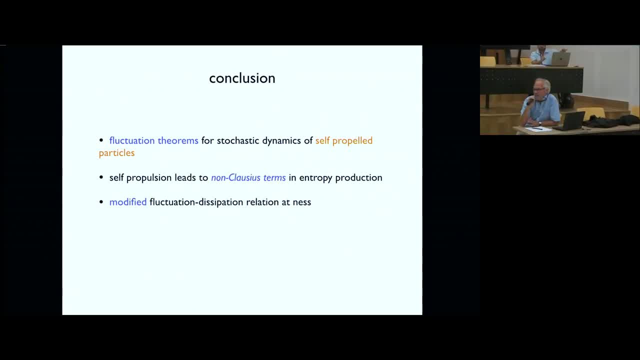 you will typically not get the heat coming from the source energy supply, and the source energy supply, from the source energy supply- doesn't actually have the energy supply- heat, for instance- which would come from a real physical process. So, in any case, I mean, we're used to play these games now. 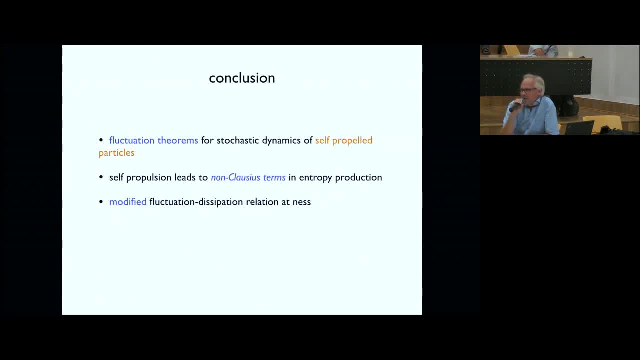 for 10 or 15 years. But if we do it for these cost-grade models, we should accept the fact that we get something, but it's not necessarily what you would call physical entropy production. Yeah, Any other questions? Yeah, So when you look at the response here, 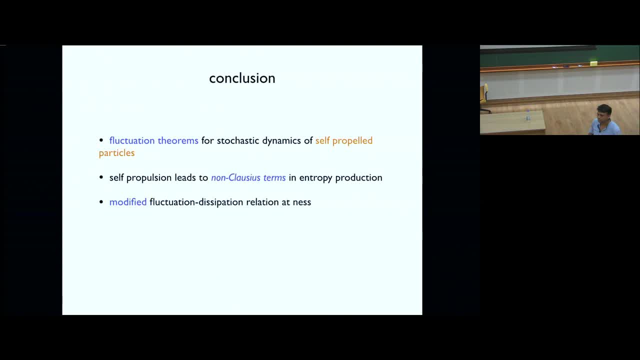 it's sum of two parts, right? I mean, can you say how it compares with this formalism of Christian Meisertal, where they also have this response in? So this sum of two parts- here are the correlation of the one part is nonlinear in velocity. 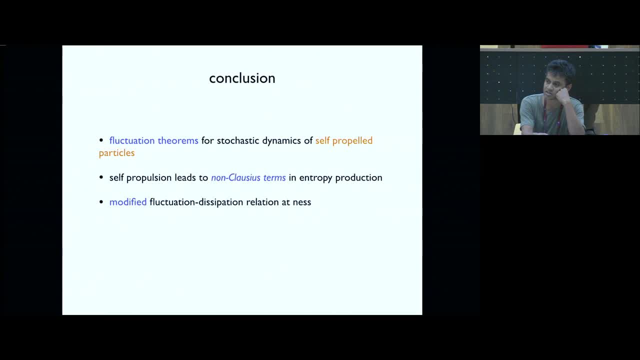 One function is nonlinear in velocity, So this nonlinear velocity function times the normal velocity term. So this nonlinear part g of v at time t and v at time 0.. And then the other part is actually just reverse of that v at time t with g of v at time 0. 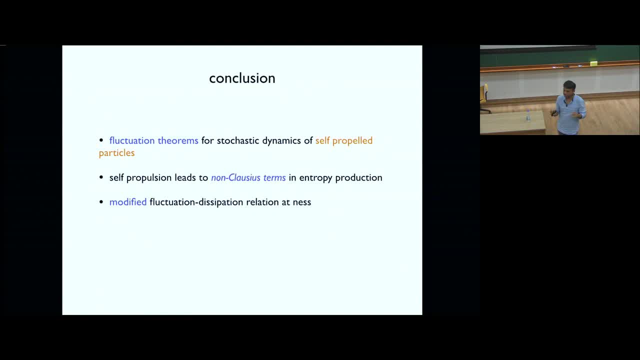 So these two terms, then once you make them both linear, then they are equivalent to each other, Then they add up and gives rise to the normal fluctuation dissipation relation. what we know, But this guy is because it's a nonlinear term.